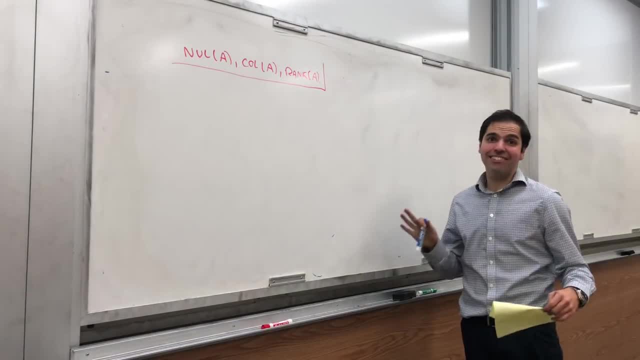 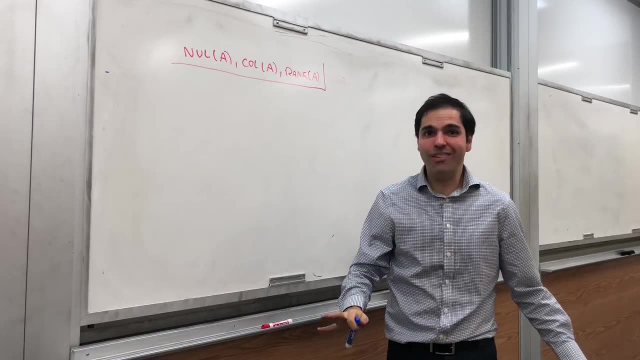 All right, thanks for watching And I don't wanna say this video is important. but this video is super important, especially if you're cramming for a linear algebra exam and you have one in an hour or something and you need to know all the concepts. 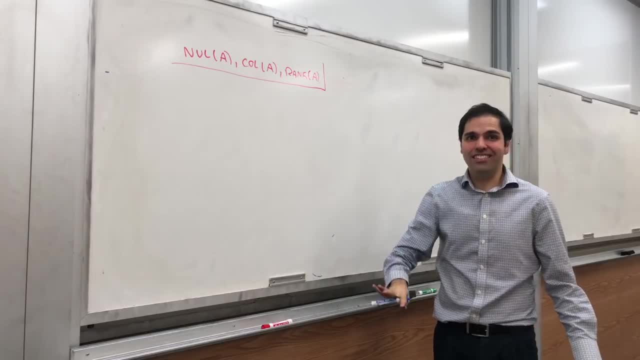 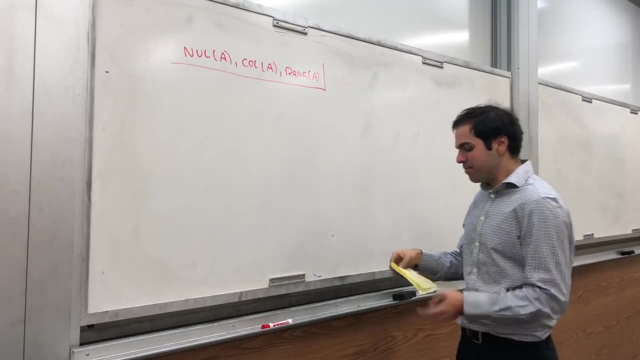 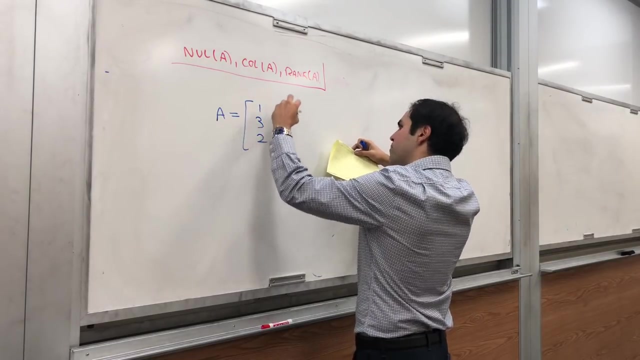 Well, turns out, this one problem has all the concepts in it, or at least most of them. so make sure to watch it. I'm not even exaggerating. So, in particular, let's take this matrix here: A is one, three, two. 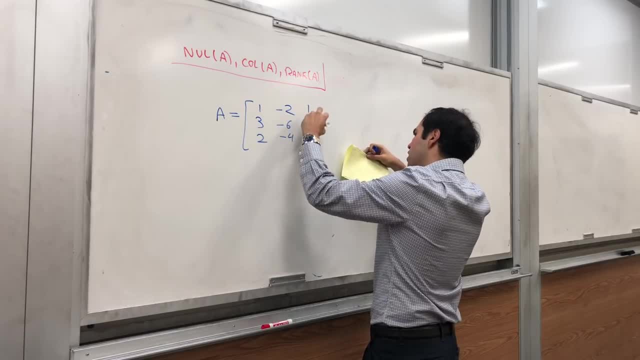 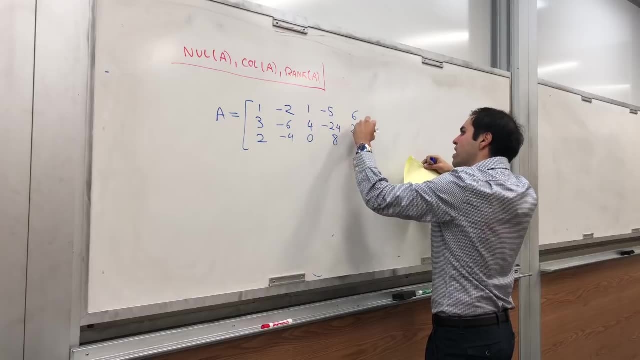 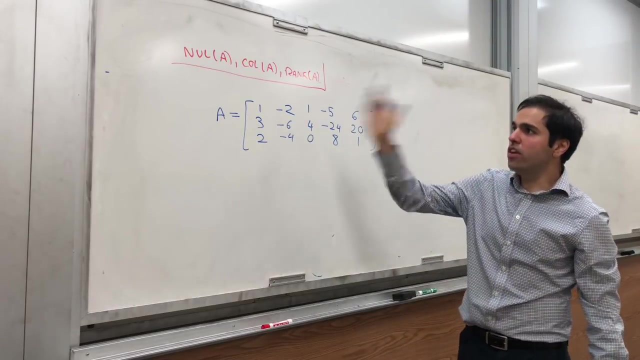 minus two minus six minus four, one four, zero minus five minus 24,, eight and six, 20, and one. What we'd like to talk about are what are called matrix spaces, So null space of A column, space of A. 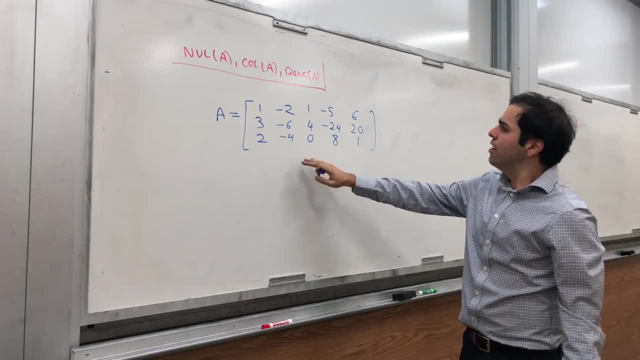 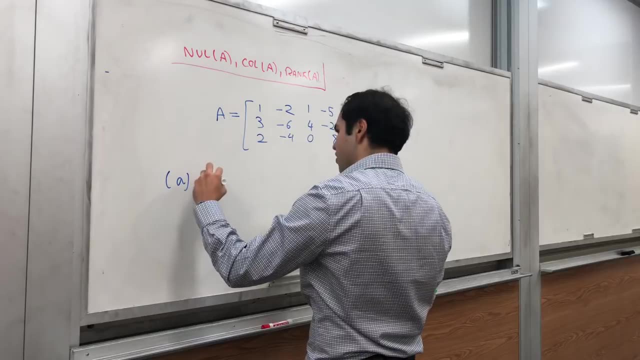 and maybe others if I have time. In particular, let's consider this matrix And first of all, let's find a basis for the null space. Oh sorry, not null space, column space. first, Find a basis for the column space. 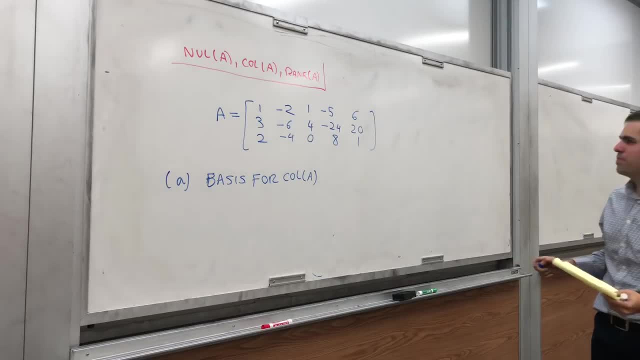 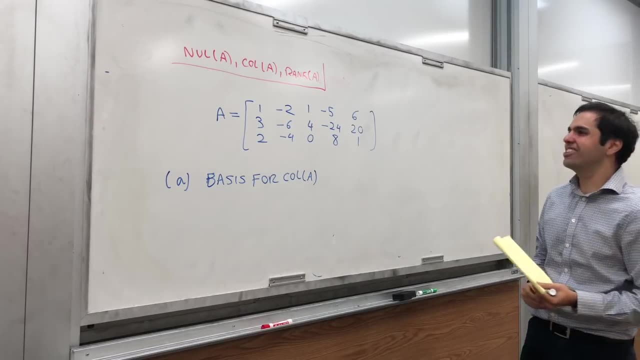 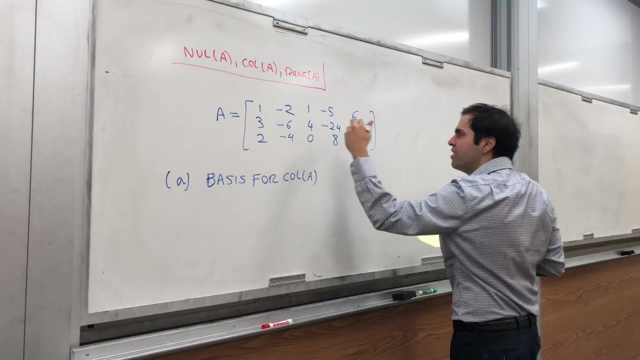 because it's a bit easier to find a basis for the column space. And in order to do that, let's row reduce this matrix. So you know, the answer to every question in linear algebra is row reduction. So let's do that. We would like to get rid of this three and the two. 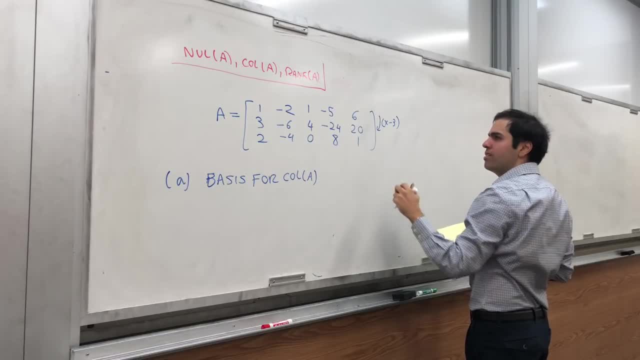 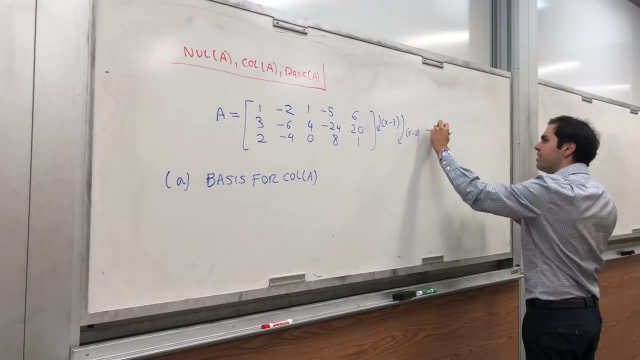 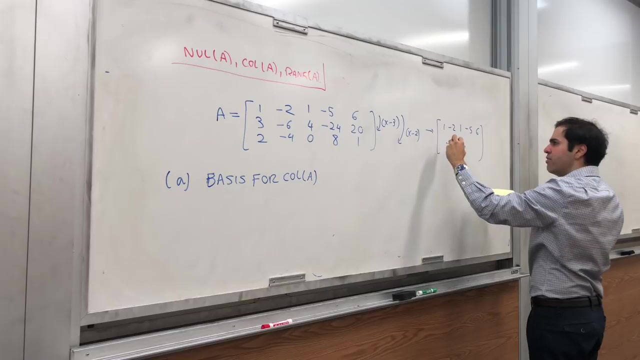 So let's subtract three times the first row from the second row and let's subtract two times the first row from the third row, And then you get one minus two, one minus five, six, And then let's see zero, zero. one minus nine and two. 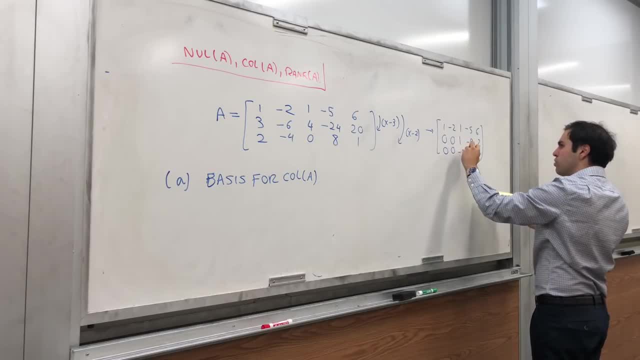 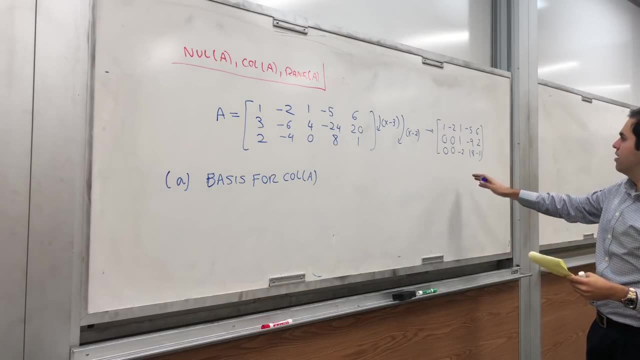 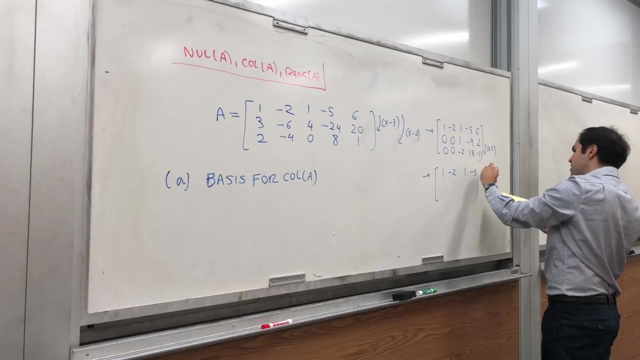 And zero. zero minus two, 18, and minus 11.. All right, almost done. So we still need to get rid of this minus two. So let's add two times of second row to the third row and we get one minus two, one minus five, six. 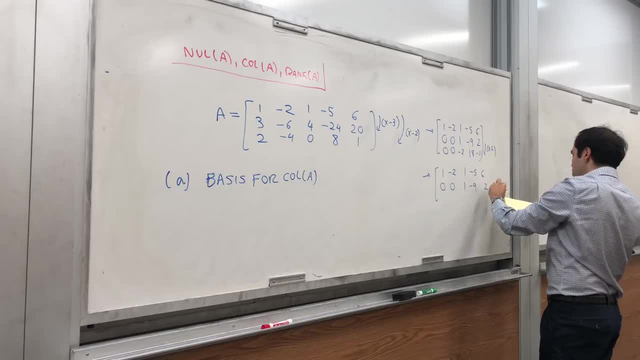 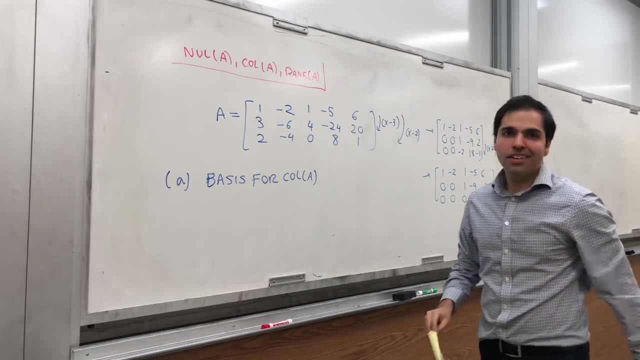 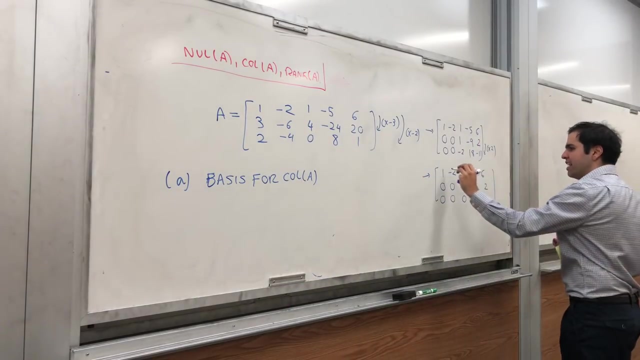 zero. zero one minus nine, two and two and 0, 0, 0, 0, minus 7.. Okay Again, any question of linear algebra boils down to row reducing and also finding the pivots. 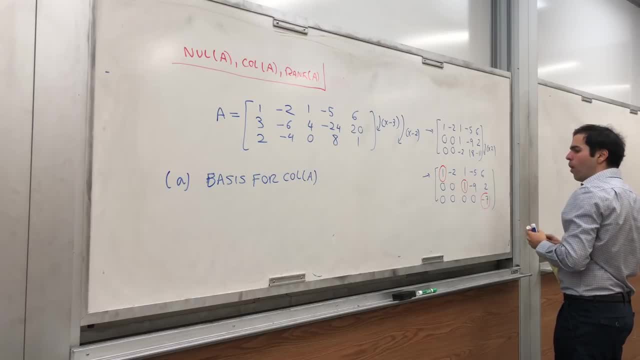 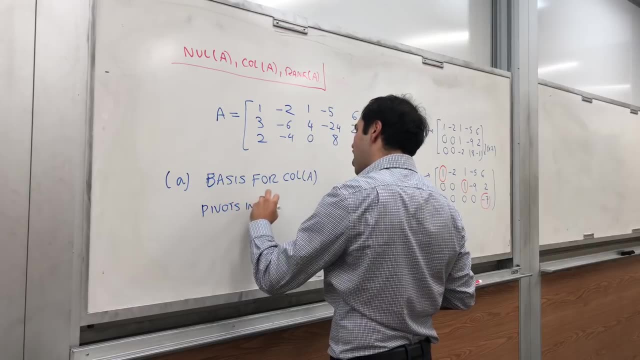 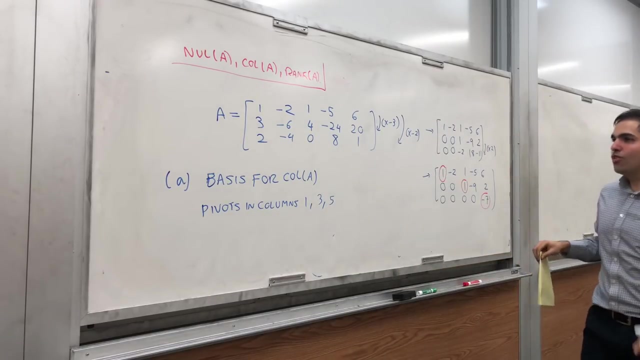 Notice. here there are three pivots: 1, 1, and minus 7.. In particular, your pivots in columns 1,, 3, and 5.. Now to find a basis for the column space of A very important 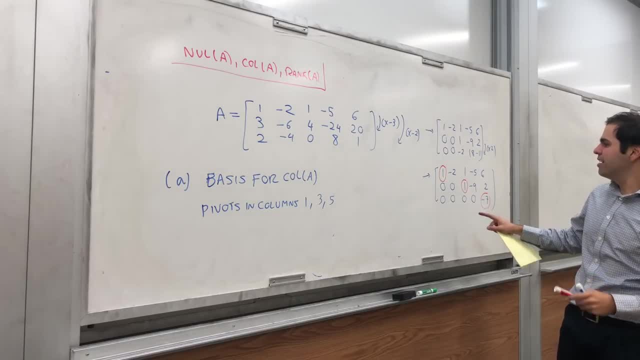 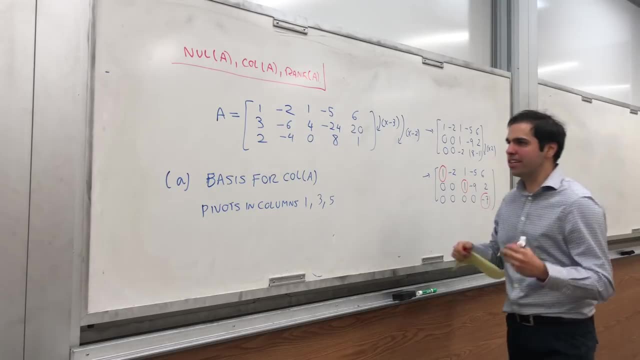 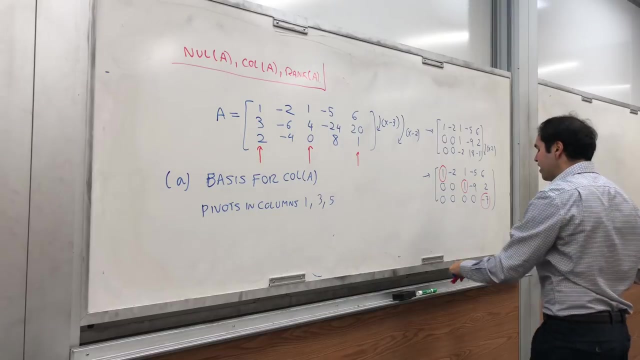 number one mistake people do in those kinds of problems. you're not allowed to choose those three things. You have to go back to your original matrix and pick the first, First, third and fifth columns of A. And the reason for this is: 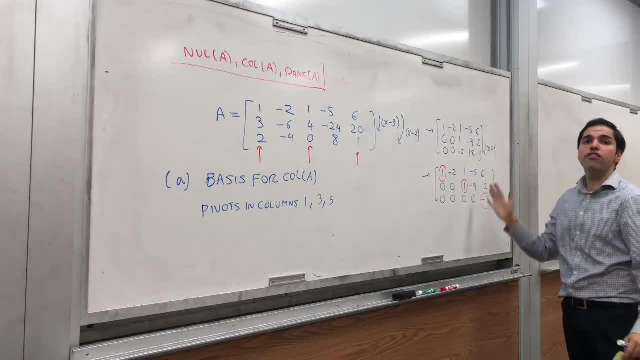 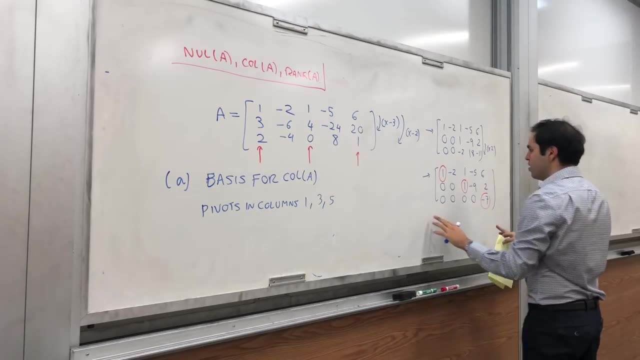 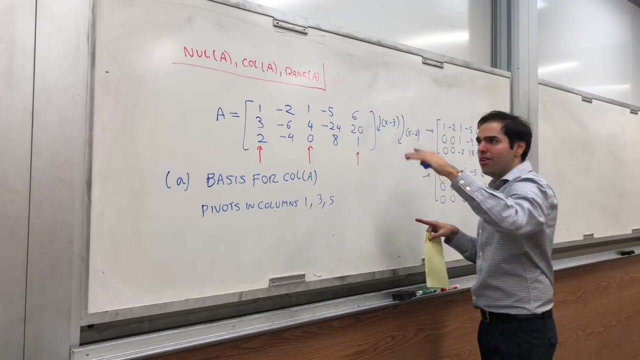 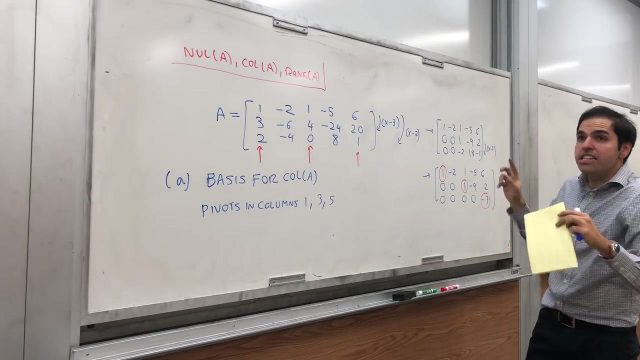 turns out row reduction, they preserve linear independence. So, vaguely speaking, if you row reduce, notice those three vectors are linearly independent. Therefore we also get that those three vectors are linearly independent. So we have those three linearly independent vectors. 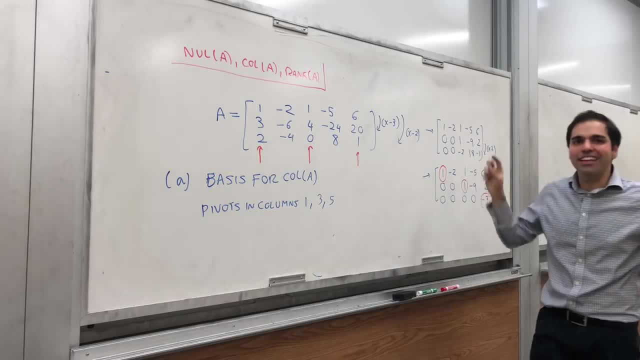 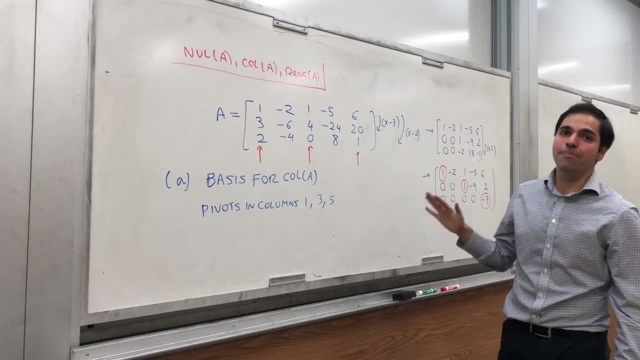 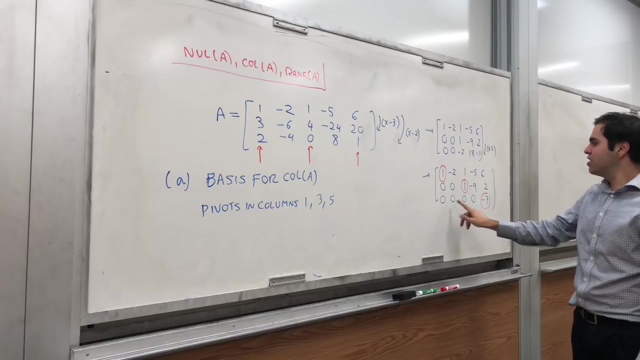 and those are automatically linearly dependent. And I put quotation marks because technically a set is linearly independent or dependent, not vectors. However, row reduction destroys the span, So the span of those three vectors is not the same as the span of those three vectors. 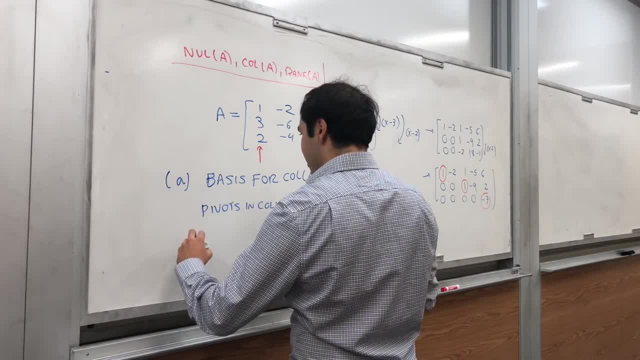 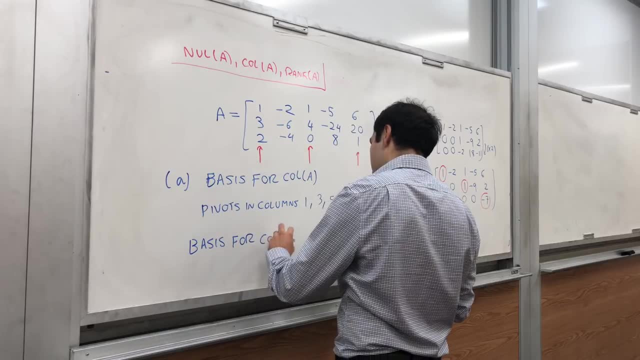 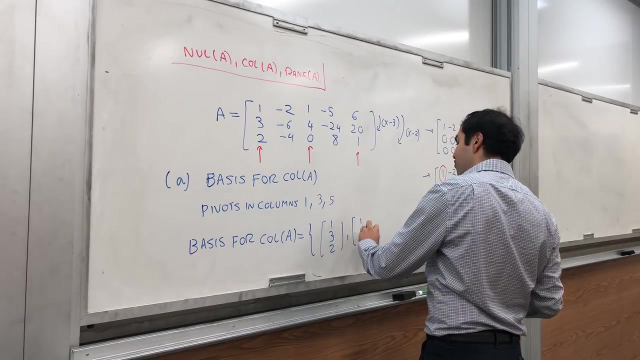 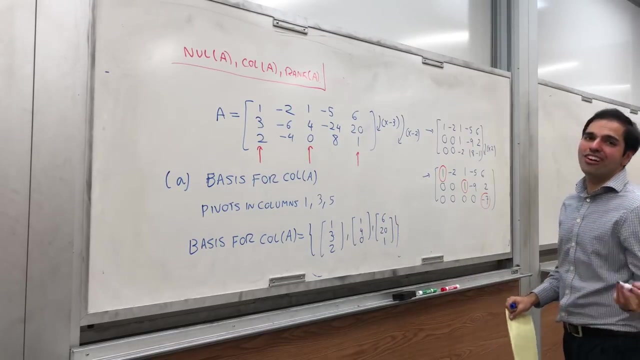 So, in particular, the basis for the column space of A is 1,, 3,, 2,, 1,, 4,, 0, and 6,, 20, and 1.. And I totally forgot to say what is a column space. 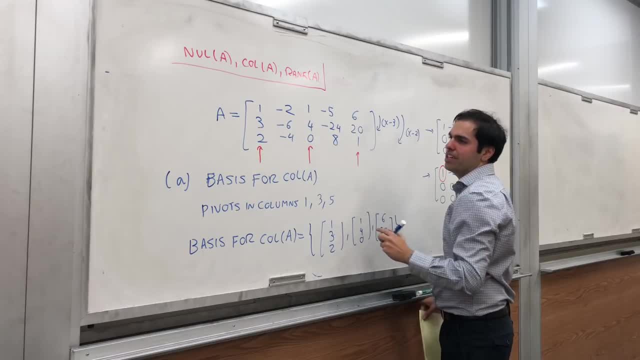 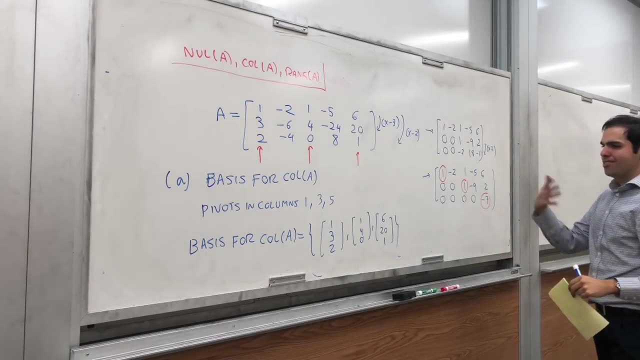 It's just the span of the columns of your matrix. So it's the span of this vector, this vector, this vector and this vector. But, in particular, a basis for the column space is that. And question: what is this a subspace of? 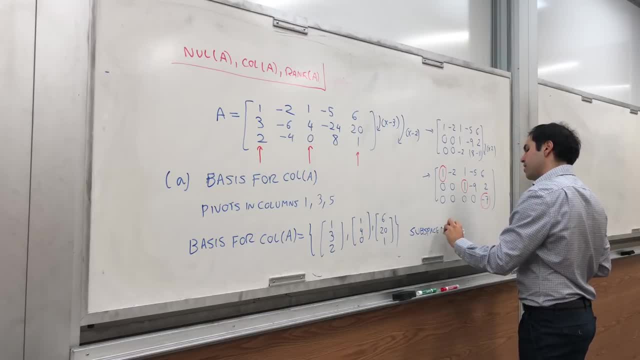 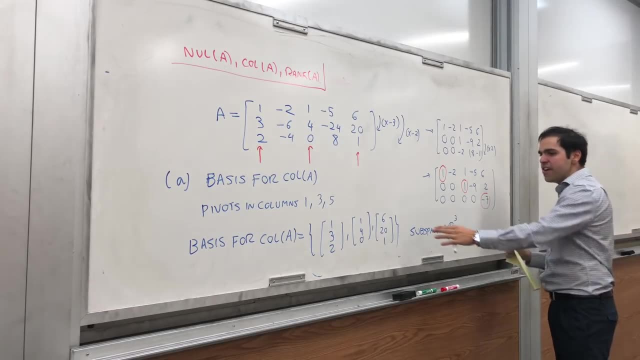 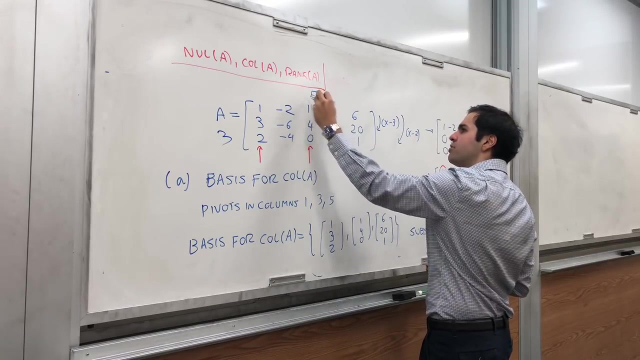 Well, here it's a subspace of R3.. So remember, subspaces are nice spaces And here they're subspaces of R3.. And notice precisely, A is a 3 by 5.. It's a 3 by 5 matrix. 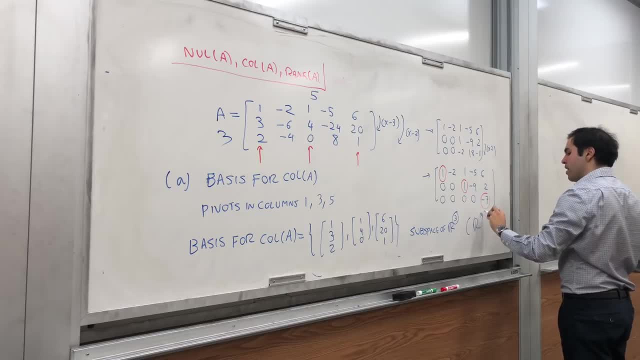 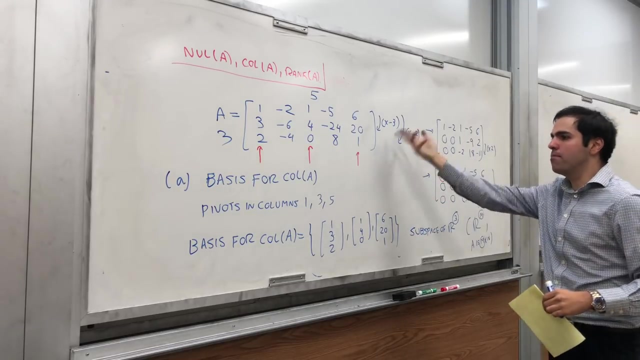 So in general, it's a subspace of Rm, where A is m by n And I like to think of it in terms of input and mouthput. So column space deals with outputs, with mouthputs, Or another way to remember this. 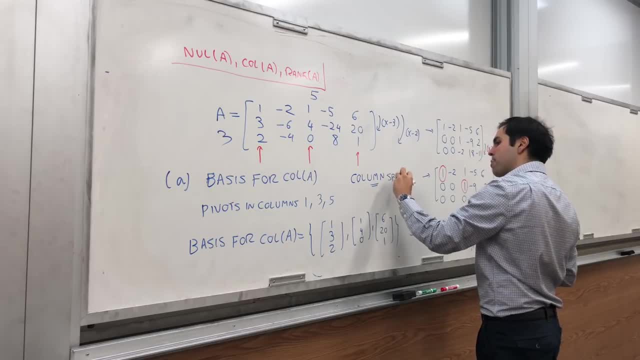 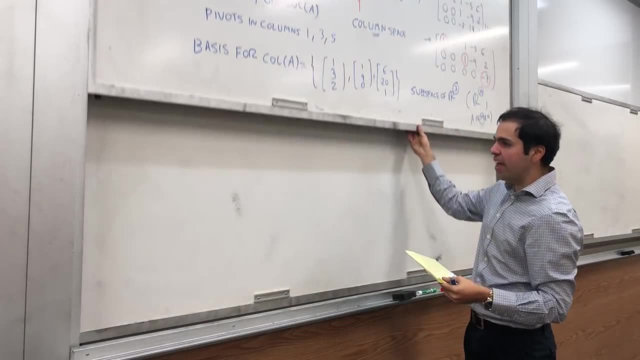 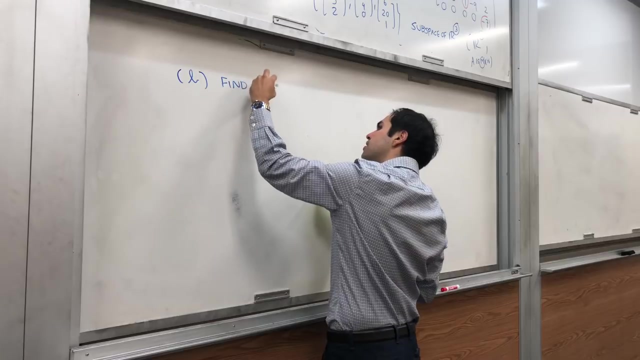 we have column space M, as in column. Okay, That's one thing. So the basis for the column space of A. Then the second thing is find what's called the rank of A. All that rank of A is is just a fancy word. 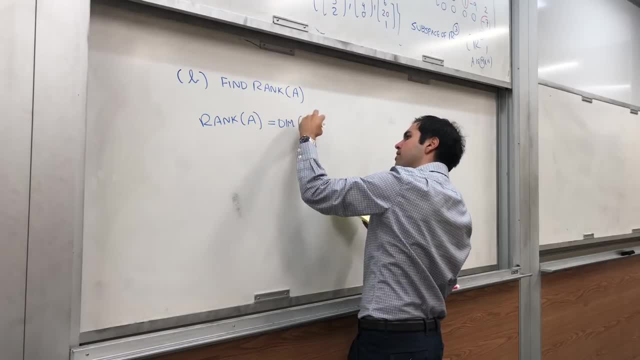 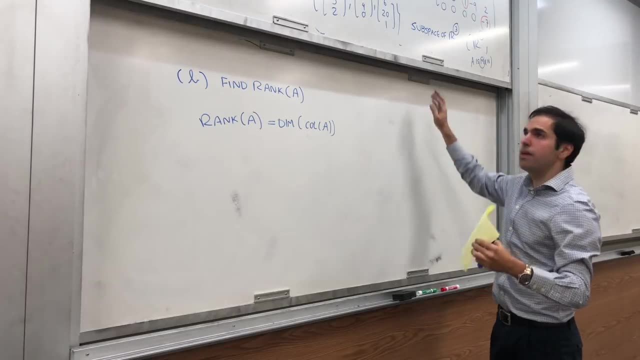 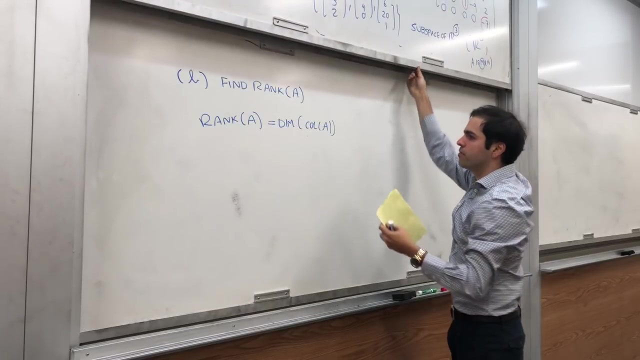 for the dimension of the column space. How do you find the dimension? Just count the number of vectors in the basis. So here there are three vectors in this basis. So the dimension is 3.. That's 3. And it turns out. 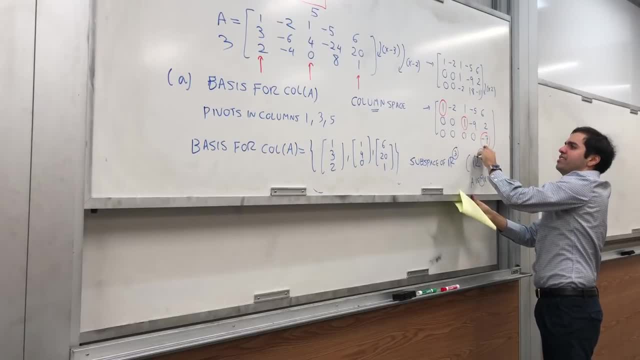 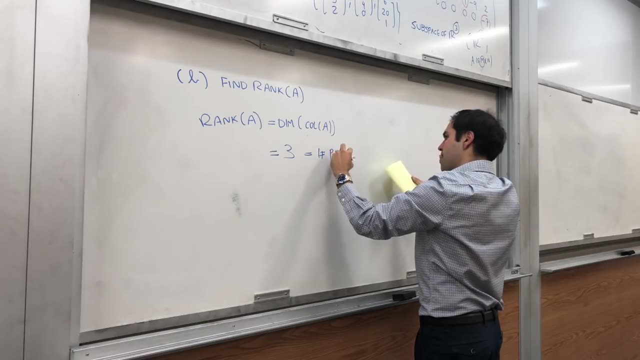 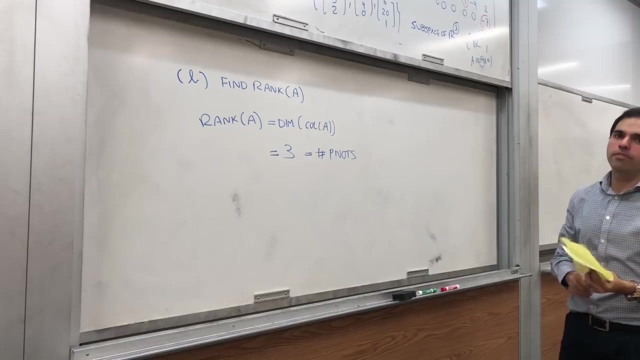 it's exactly equal to the number of pivots here. So we have three pivots, So the rank is 3.. And sort of the rank tells you how good a matrix is. The bigger the rank, the better the matrix. 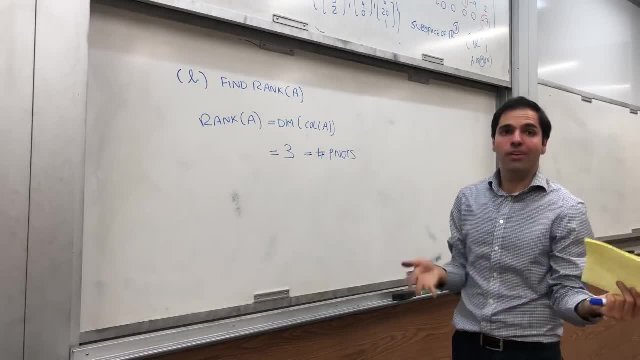 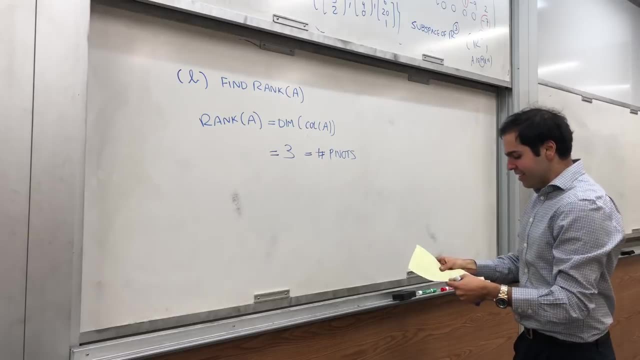 For example, the 0 matrix has rank 0. It tells you nothing, But the identity matrix has the highest rank possible. All right, So that's one thing. And then let's find. on the one hand, we found the column space. 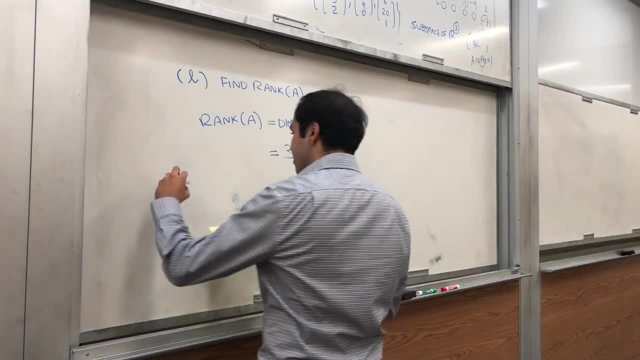 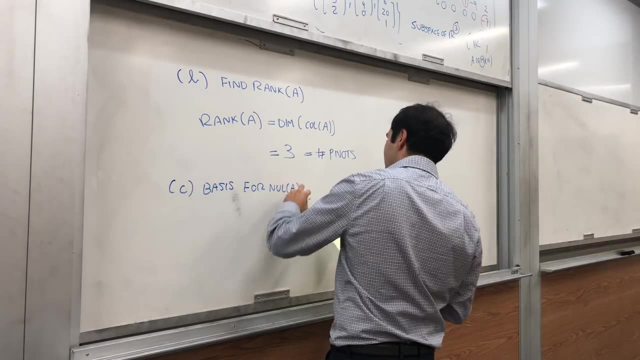 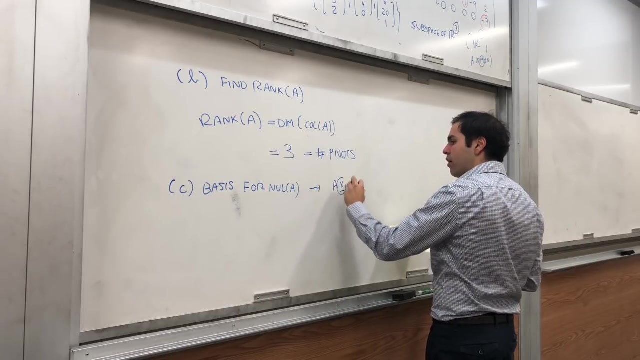 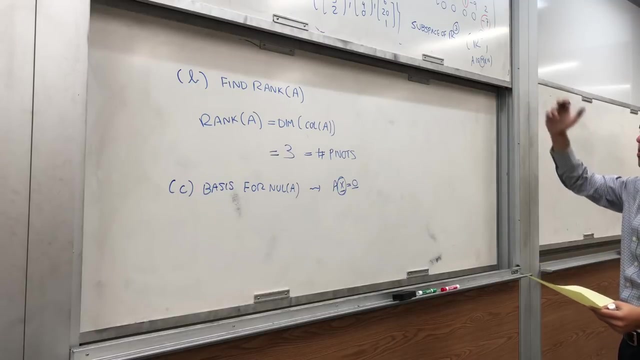 Now let's find the basis for the null space, For null of A And again null of A. that's just the set of solutions of. Ax equals 0. Which means you have to find x, Very important. The column space deals with the outputs. 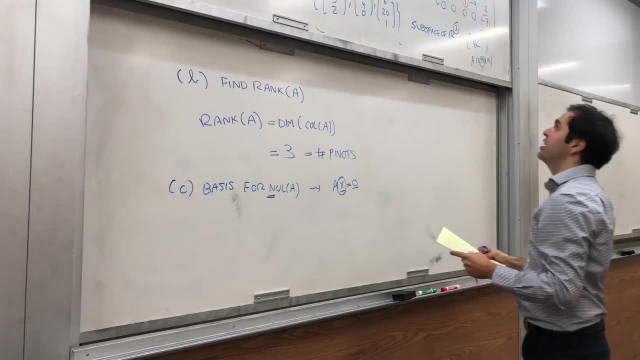 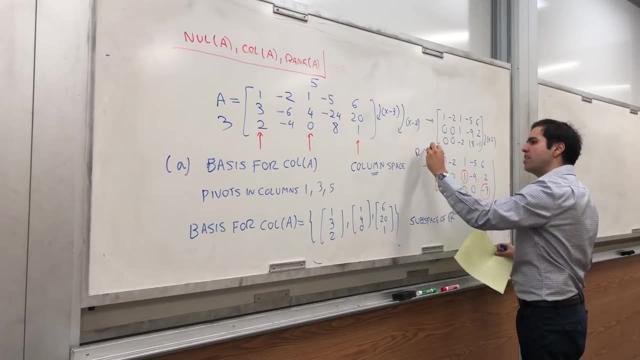 The null space deals with inputs. That's our young And, but that's good. In order to do that, well, we row, reduce the matrix to the row echelon form. But to find the null space you need to go one step further. 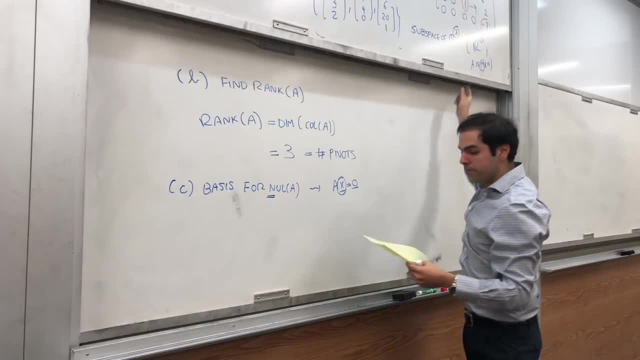 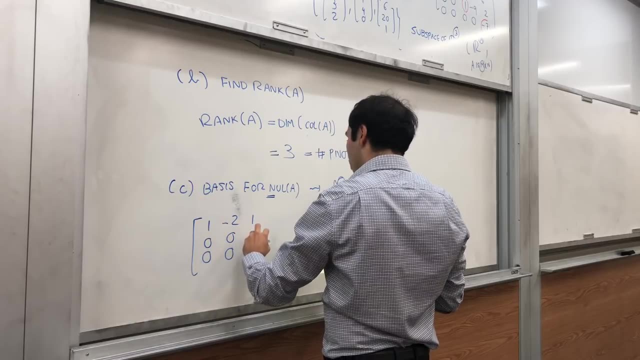 and do the reduced row echelon form. So let's start with this. So 1, 0, 0.. Minus 2, 0, 0.. 1, 1, 0.. Minus 5, minus 9, 0.. 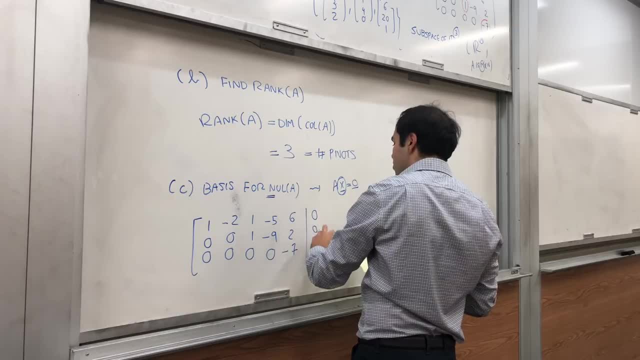 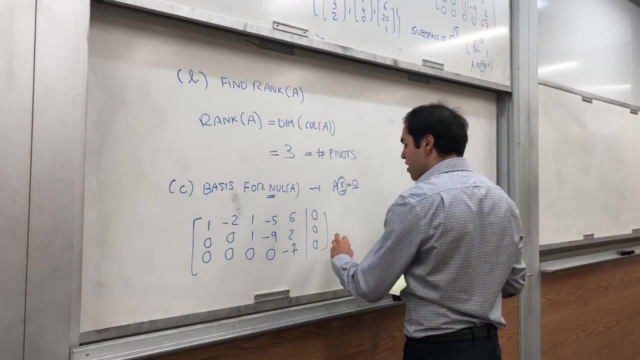 6,, 2, minus 7.. And then want to solve: Ax equals 0. So we put a bunch of 0s here, And then you want the reduced row echelon form, which first of all means the pivots have to be 1.. 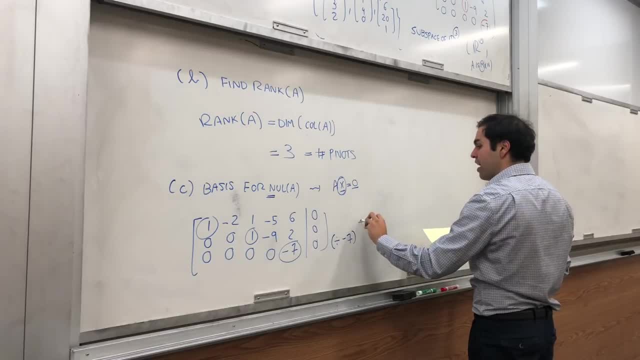 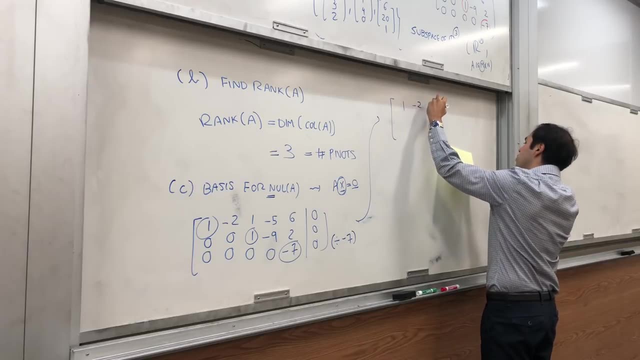 So turn this minus 7 into a 1, and we get maybe over there. We get so 1, minus 2.. 1, minus 5, 6. 0, 0, 0.. 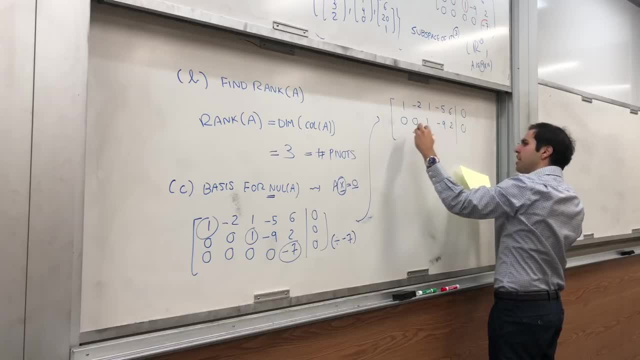 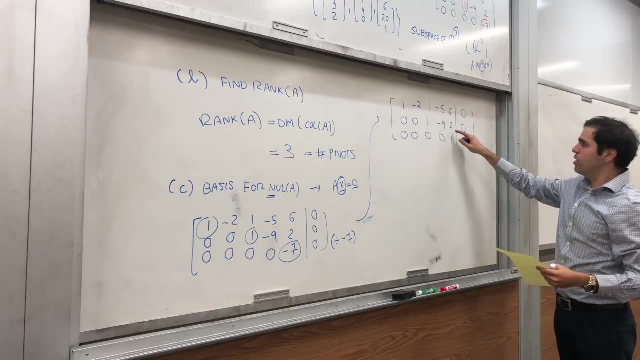 1, minus 9, 2, 0. And then 0, 0, 0, 0, 1, 0. Then next thing is we want to turn those numbers into 0s. 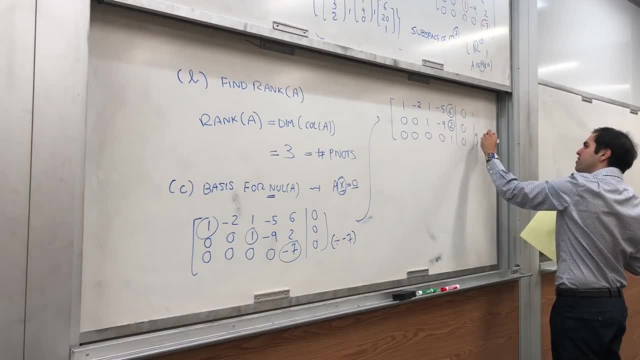 So the numbers above the numbers, the pivots, have to be 0.. But that's not too bad. Let's subtract 2 times the third row from the second row and subtract 6 times the third row from the first row. 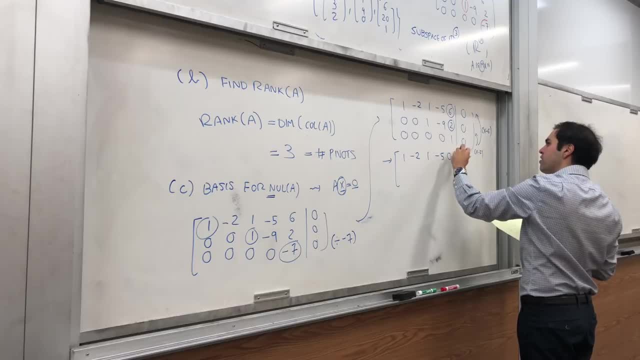 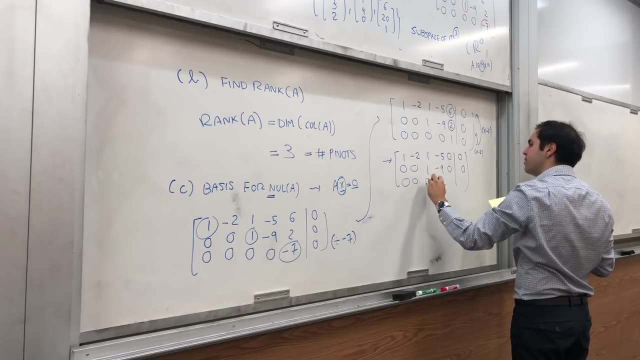 And we get 1, 2, 1, minus 5, 0, 0.. And 0, 0, 1, minus 9, 0, 0.. And then 0, 0, 0, 0, 1, 0. 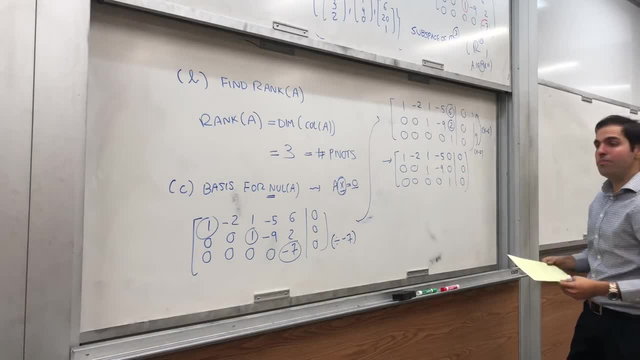 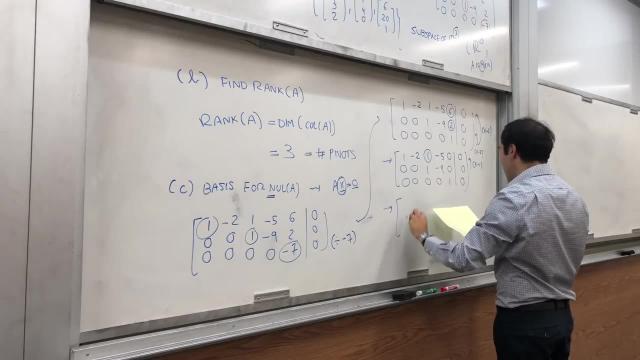 Next, we want to turn this non-pivot into 0. So let's just subtract the second row from the first row and we get 1, minus 2, 0, 4.. 0, 0.. 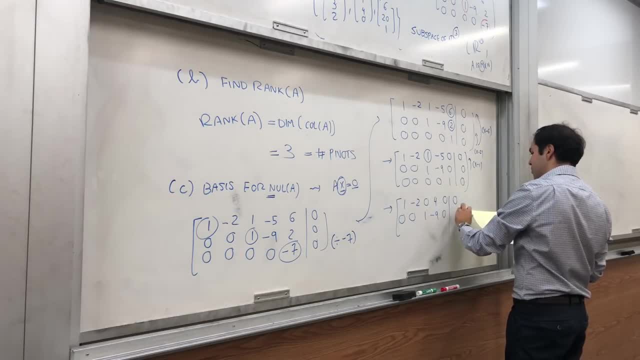 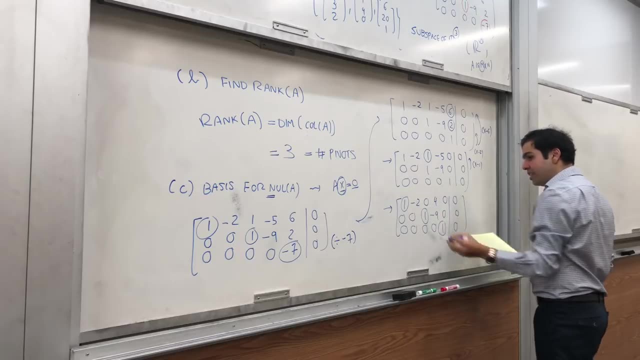 And then 0, 0, 1, minus 9, 0, 0.. And 0, 0, 0, 0, 1, 0.. So, indeed, it is in reduced row echelon form. 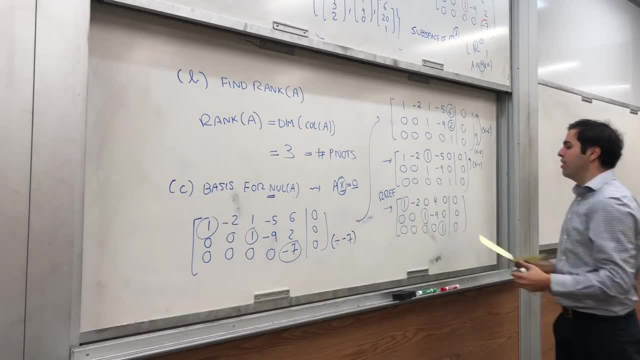 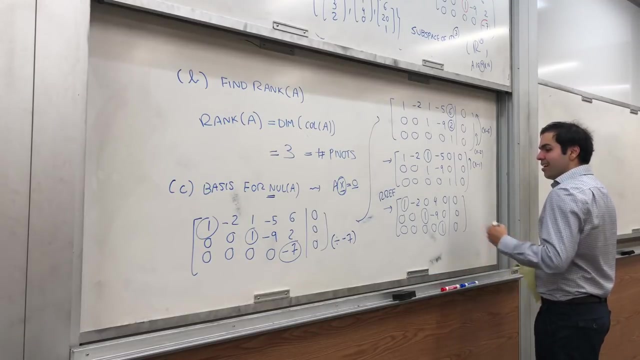 because the pivots are 1, and the stuff above and below the pivots are 0. Then let's just solve this. So one little thing. This will be very important and a thing I'll talk about next. There are pivots in the first, three and fifth column. 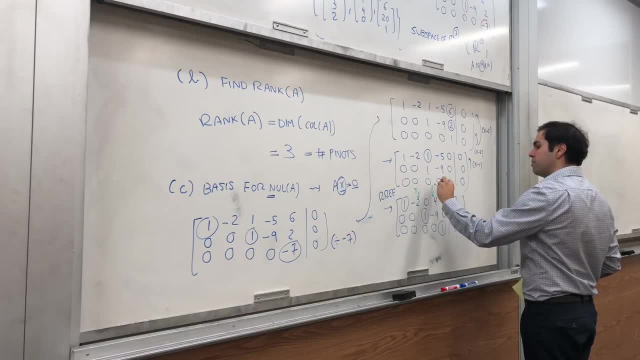 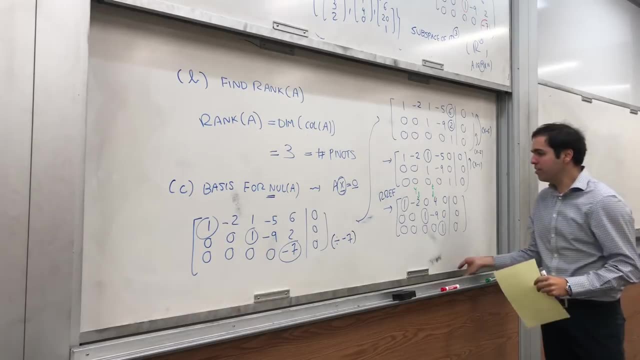 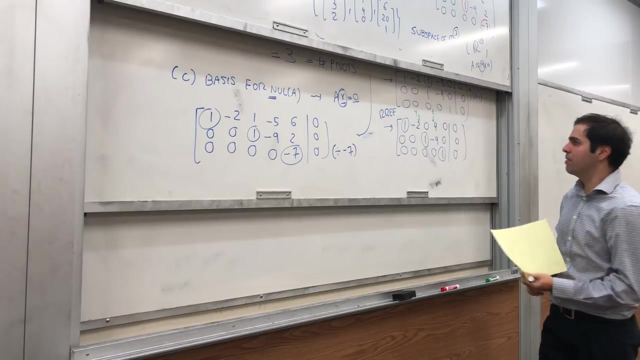 What are the free variables? They're in the non-pivot columns. So here, y and t, they're the free variables. The second and the fourth variable, And this is also very useful when you want to solve an equation before solving this, do that. 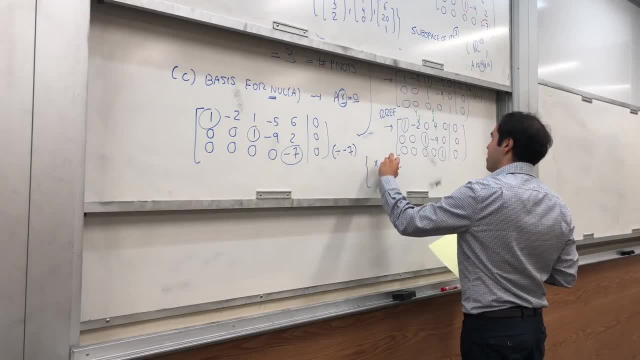 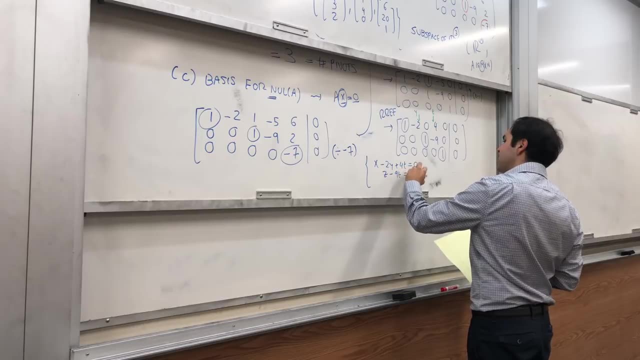 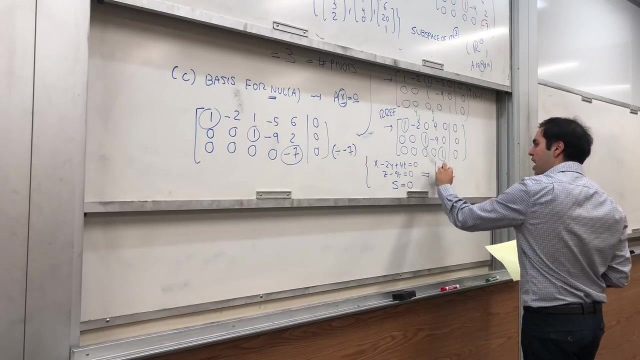 So then we get: x minus 2y plus 4t equals 0.. z minus 9t equals 0.. And the last variable equals 0. Let's call it s And then let's solve in terms of our free variables. 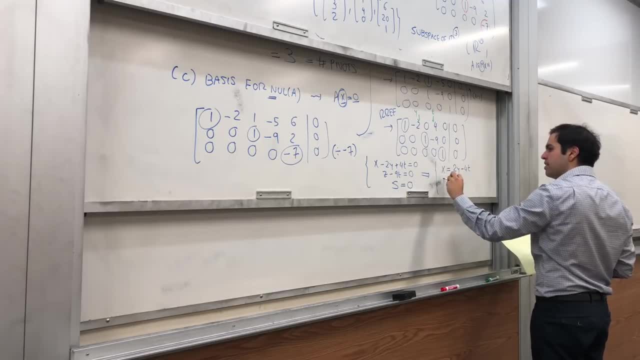 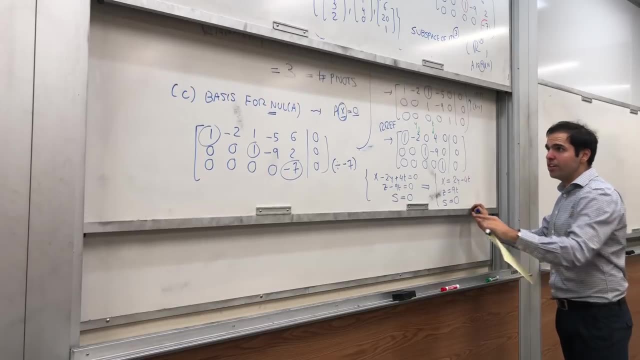 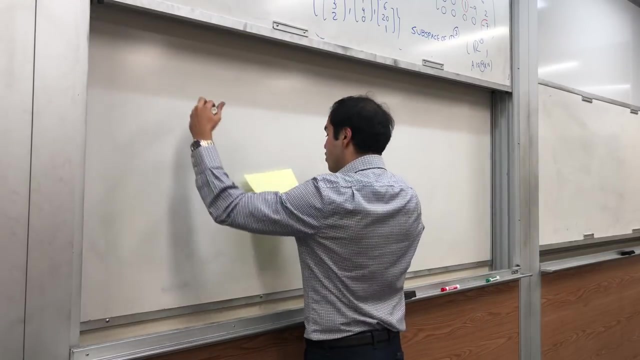 x is 2y minus 4t, z is 9t and s is 0.. Okay, why are we doing this? Because, again, we want to find x such that ax equals 0. So x then just becomes: 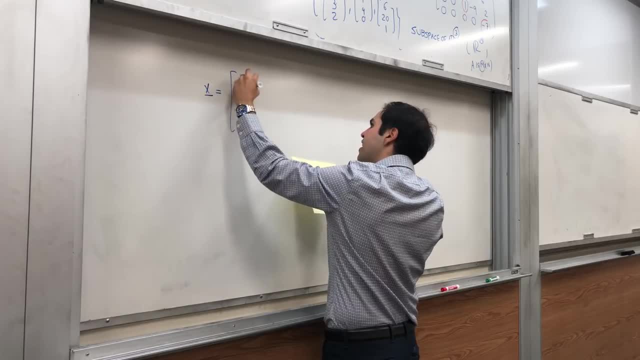 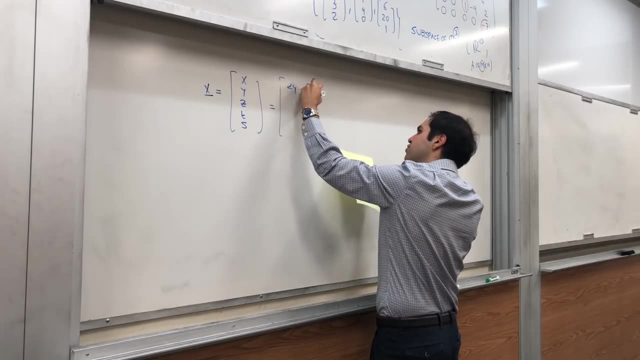 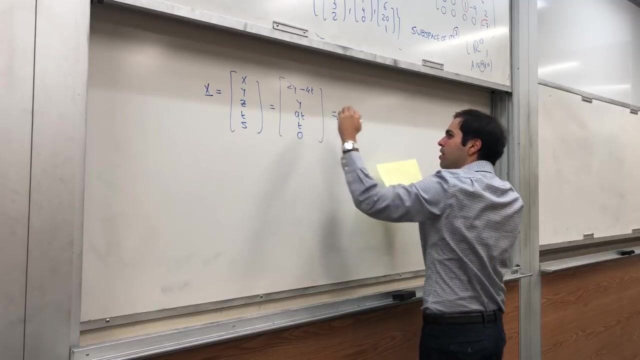 again everything x, y, z, t, s, and that becomes 2y minus 4t, y, 9t, t and 0.. And you can separate out the y's, So 2y y, 0, 0, 0,. 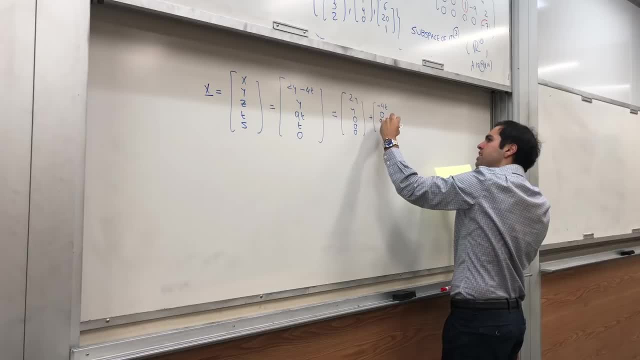 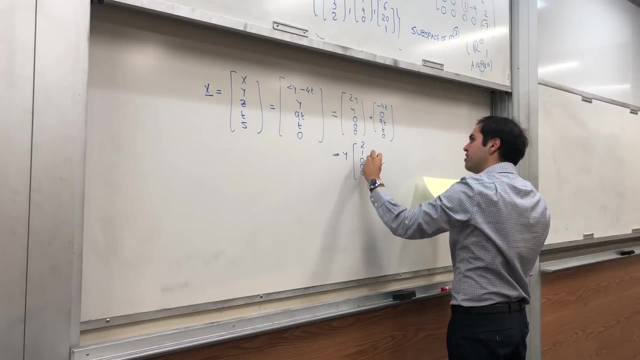 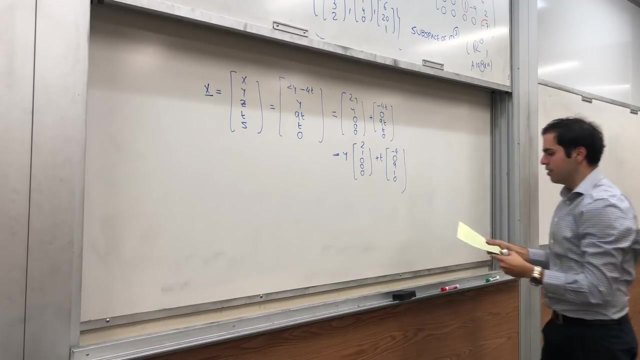 plus minus 4t 0, 9t t 0.. And you get y times 2, 1, 0, 0, 0, plus t times minus 4, 0, 9, 1, 0.. 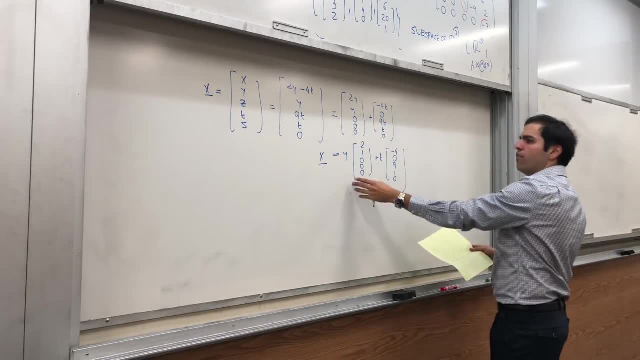 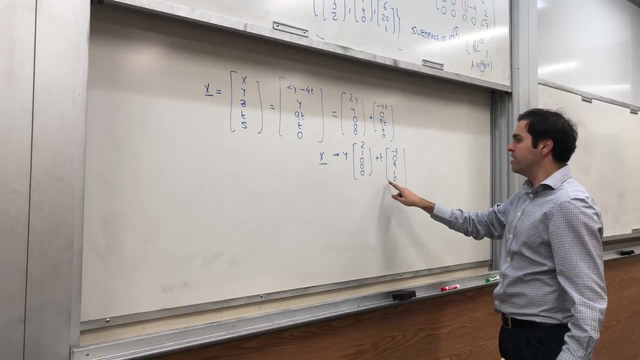 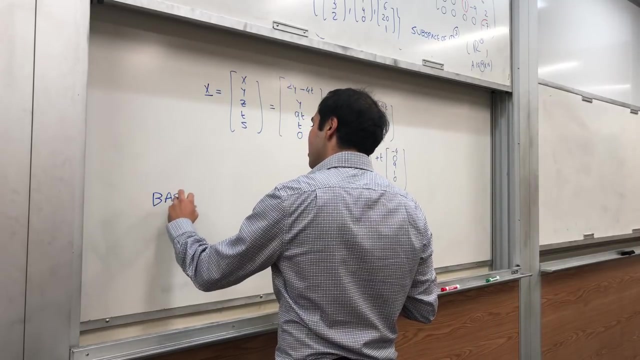 So your null space is really the set of all linear combos of those two things, And it turns out that those things will always be a basis for your null space. So the miracle of row reduction is that row reduction automatically gives you a basis. 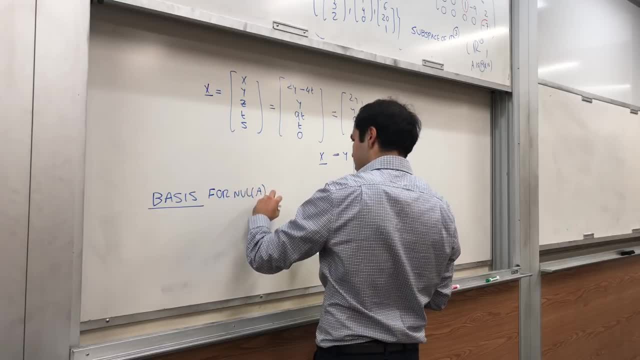 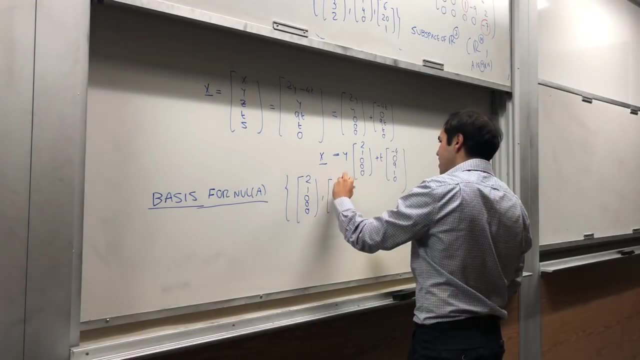 for null of A. So the basis for null of A is in this case 2, 1, 0, 0, 0, and minus 4, 0, 9, 1, 0.. 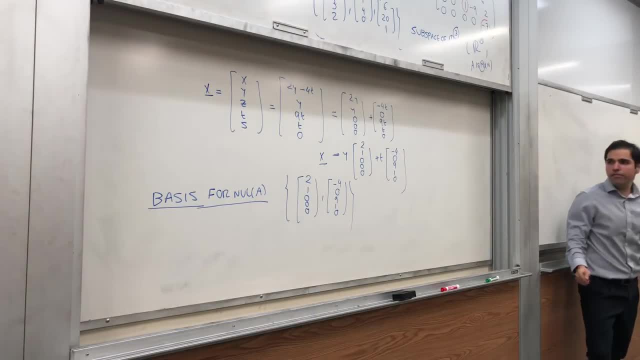 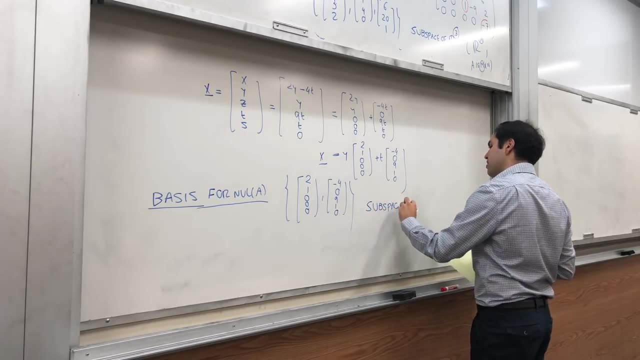 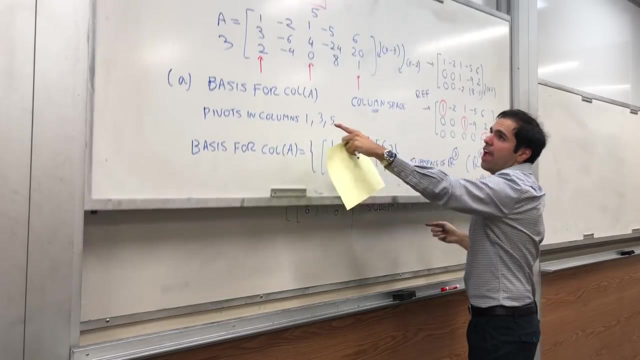 And the question is: what is this? a subspace of? Well, here it's a subspace of R5. Of R5.. Well, how does 5 relate to our matrix? For A was a 3 by 5 matrix. 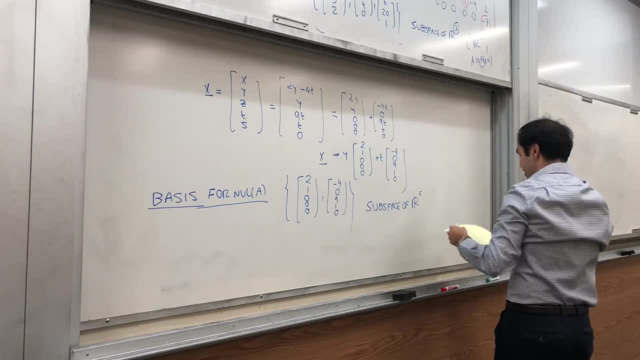 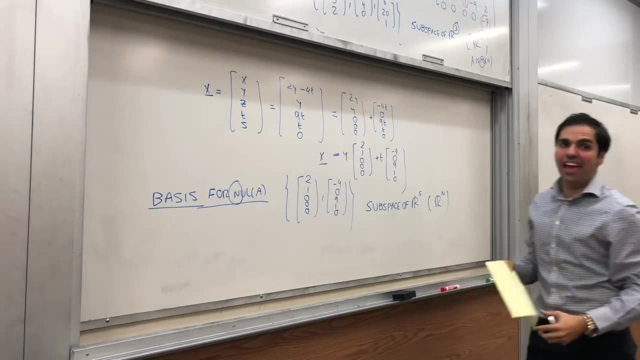 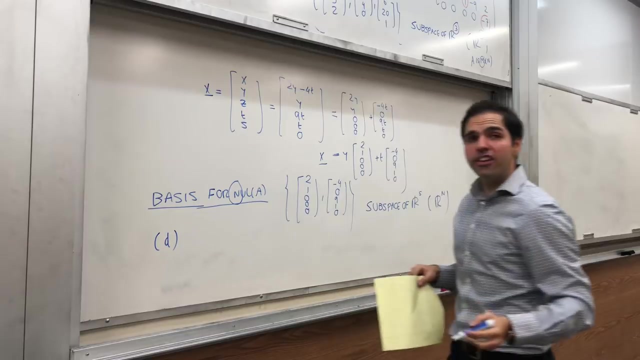 So it's in general, it's a subspace of Rn, Rn and n, as in null of A. So this is how you remember this. All right, Once we found a basis, we can find a dimension. 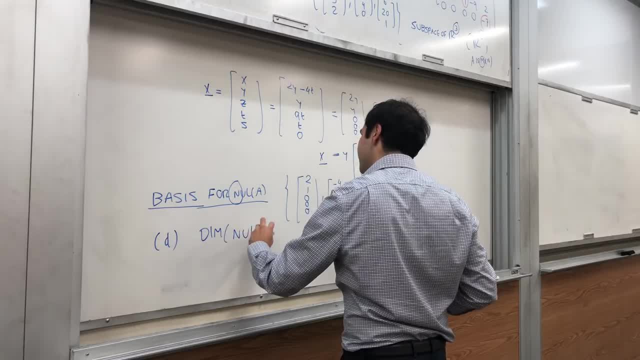 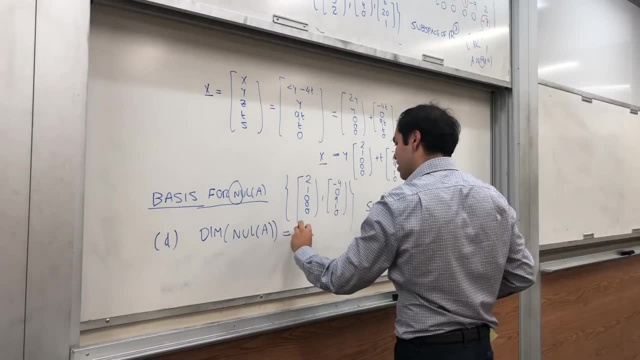 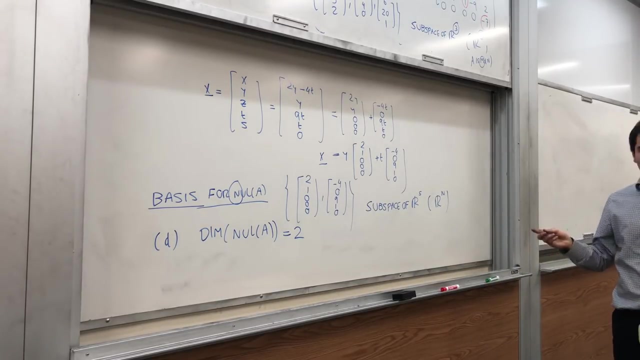 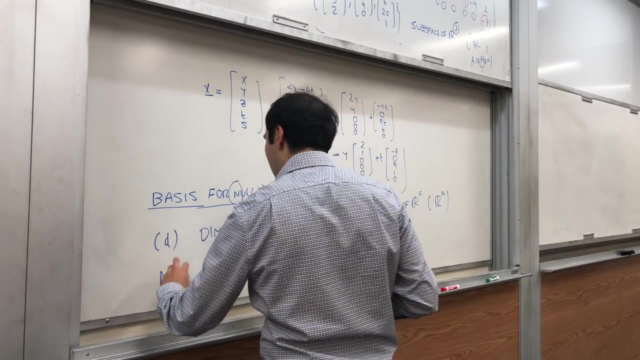 So let's find dimension of null of A. Well, you just count the number of vectors, which is 2.. Okay, Which leads us to a very important theorem in linear algebra called the rank nullity theorem. So note what happens. 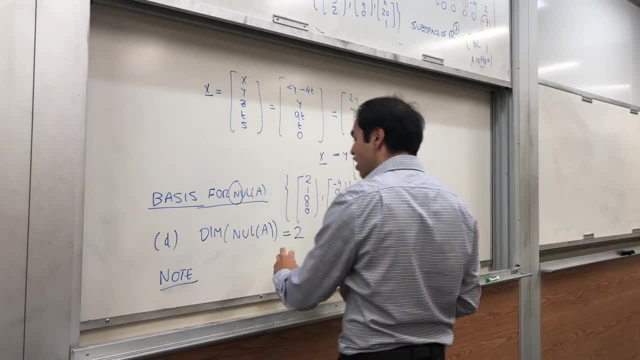 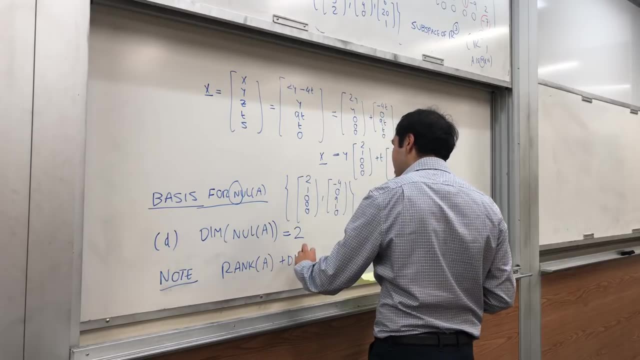 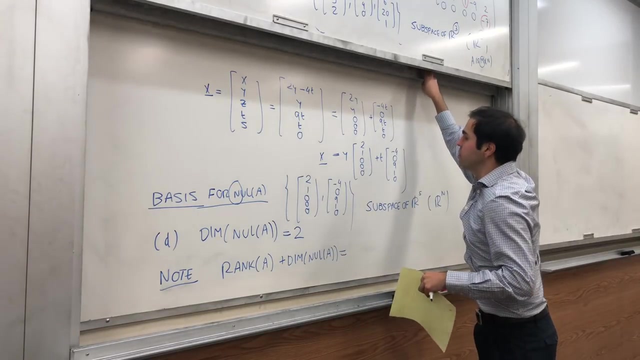 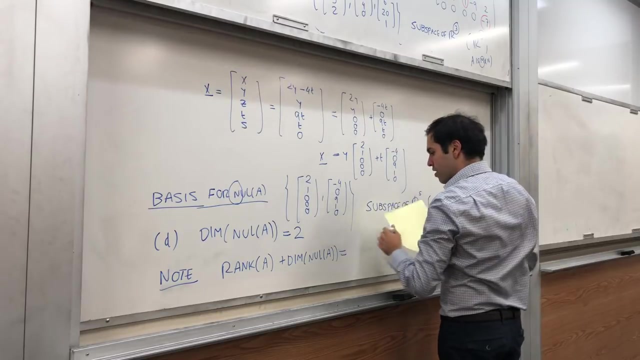 if you add the dimension of the null space plus the rank. Well, let's see: Rank of A plus the dimension of the null space of A. Rank was the number of pivots, which was 3.. There are 3 pivots here. 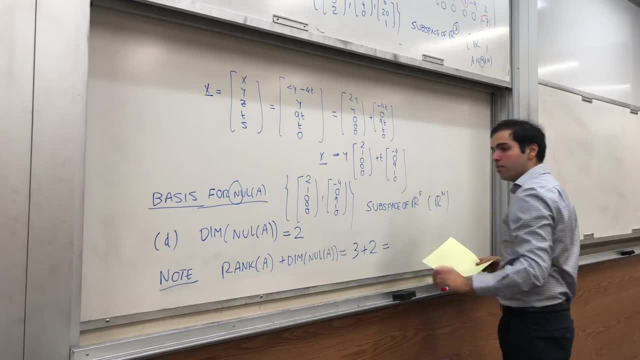 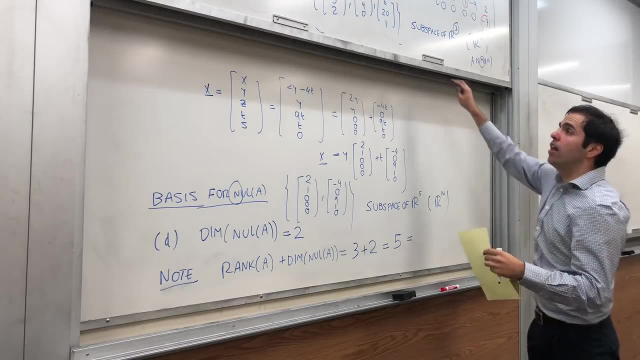 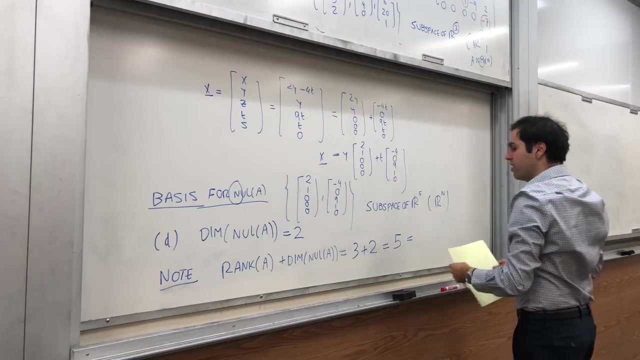 Plus dimension of null space, that's 2.. And 3 plus 2,, that's 5.. How does that relate to our matrix? Well, our matrix had 5 columns, So rank of A plus the dimension of the null space equals to n. 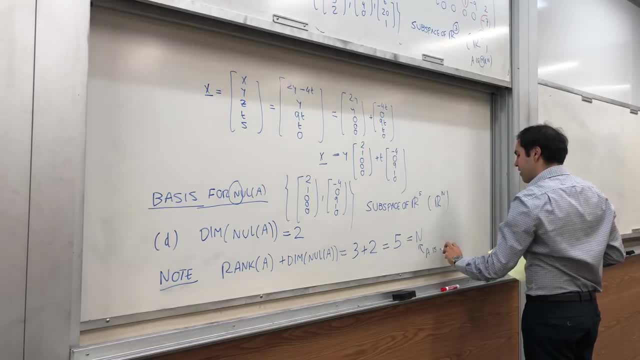 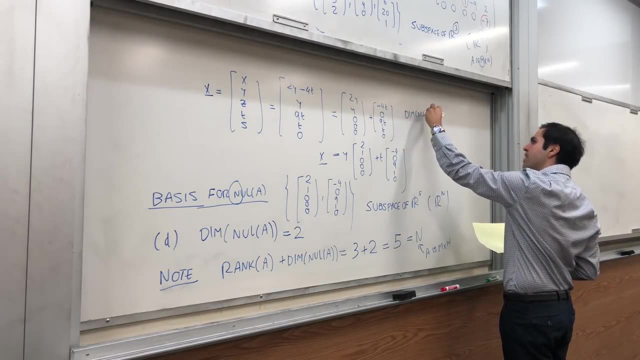 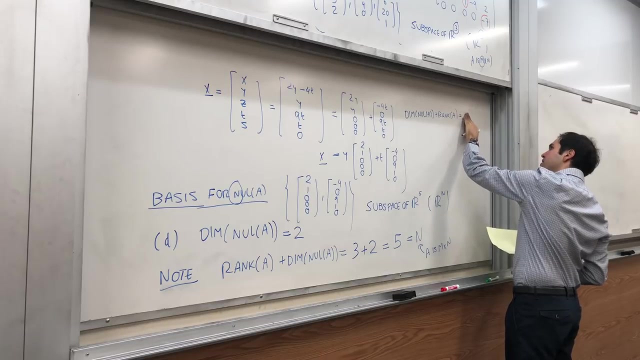 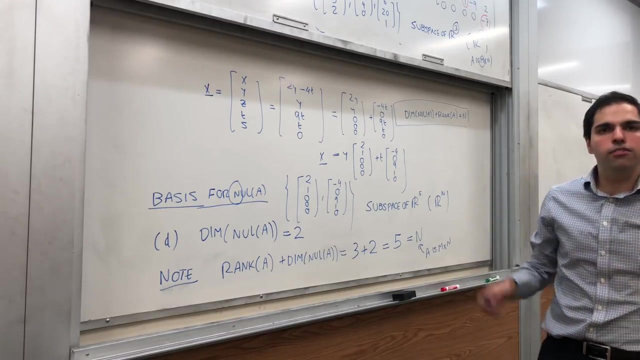 You know where A is n by n. So this is always true. It's always true that dimension of the null space of A plus the rank of A equals n. And this thing, I remember. it confused the hell out of me when I took linear algebra. 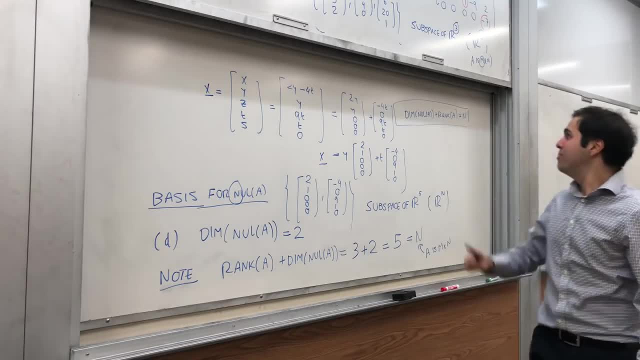 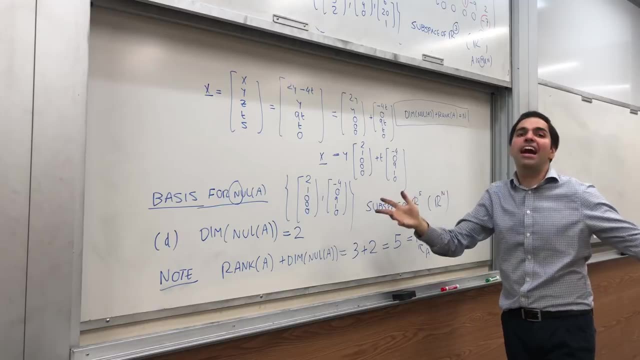 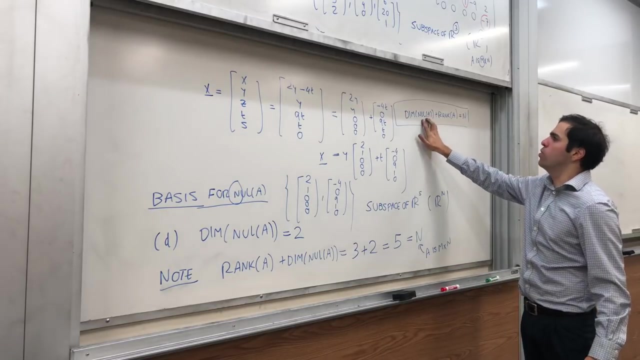 but hopefully it won't confuse the hell out of you, Because this actually makes sense. Remember: null space of A measures. how bad a matrix is? It's sort of the fat of a steak matrix or something. The bigger null of A, the worse A is. 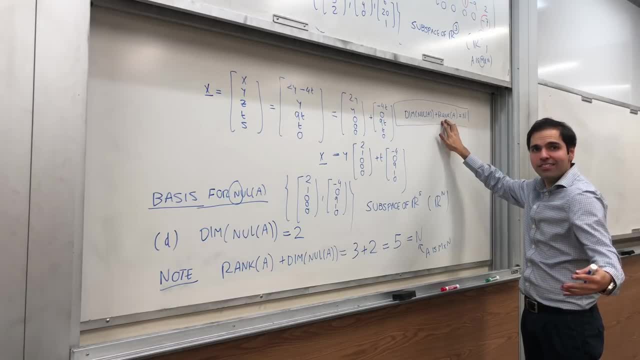 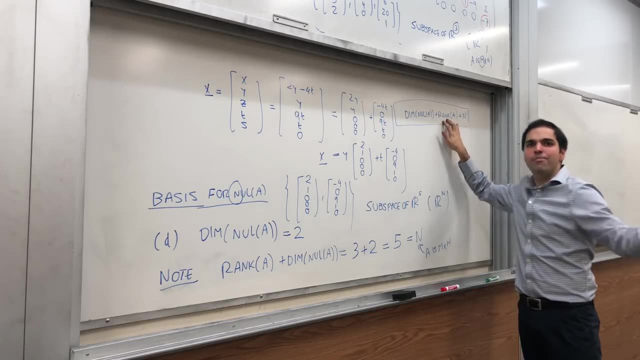 Rank, which is the dimension of the column space. The column space measures how good a matrix is, So the bigger the rank of a matrix, the better. So in other words, it's the steak part of the of a steak matrix. 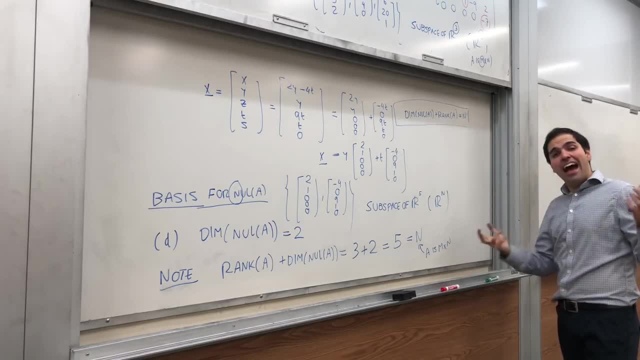 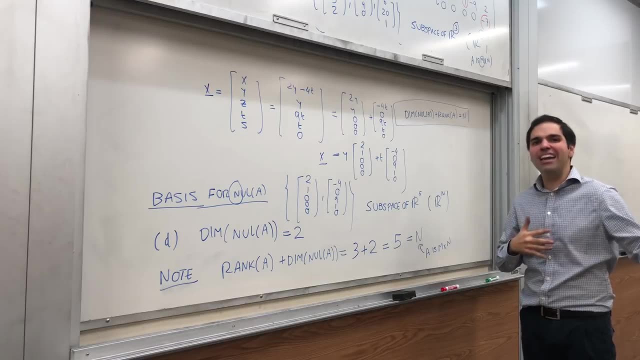 Like it's the meat part of it. Well, if you add the null space and the column space, things should balance out, Because the null space tells you how bad a matrix is, the column space tells you how good a matrix is. 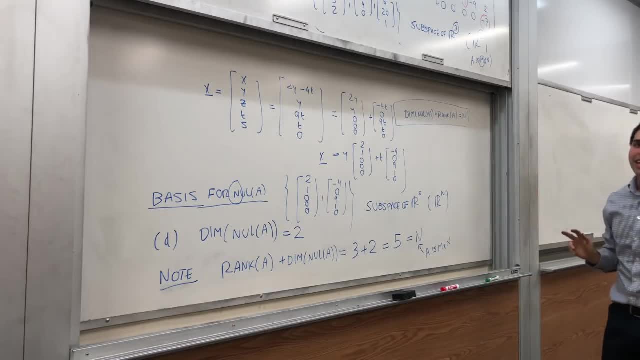 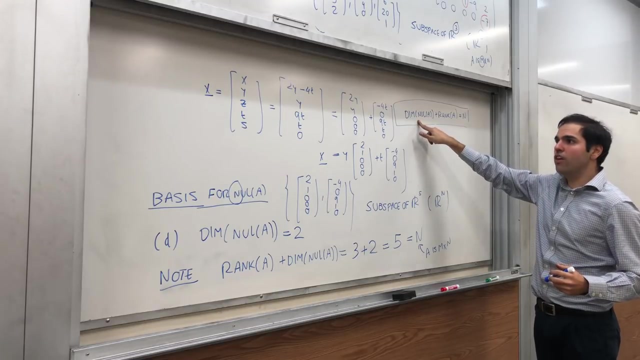 And this is precisely what this is saying here. If you add the two dimensions, then you get a fixed number, which is n. Also, how another way to figure this out? remember, the dimension of the null space of A gives us the number. 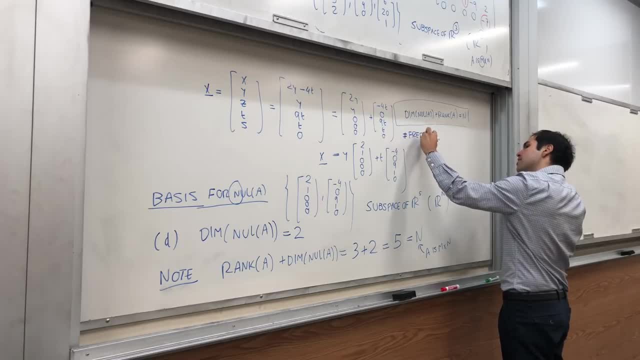 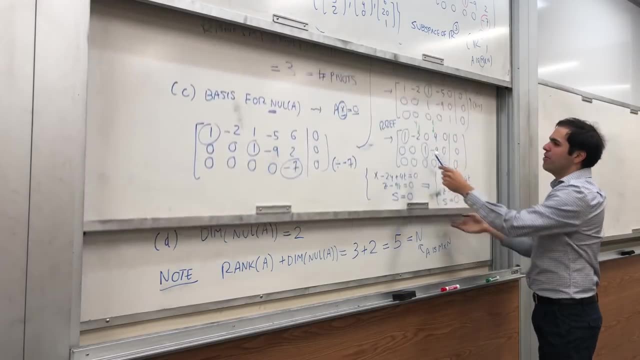 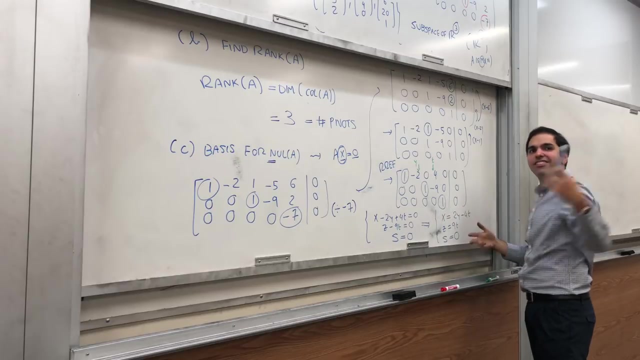 of free variables, The rank of A. you see, for example, here we had three pivots, but the free variables were in columns two and four. The pivots, they give us the non-free variable, so the prisoner variables. 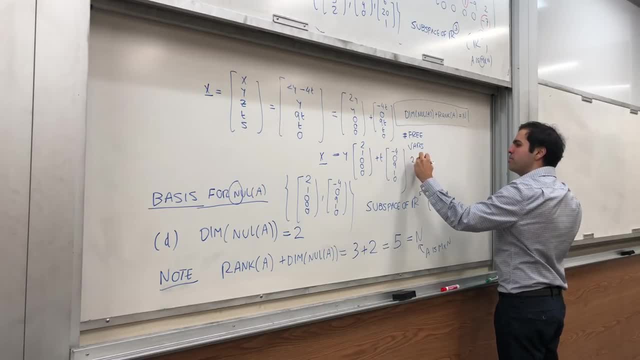 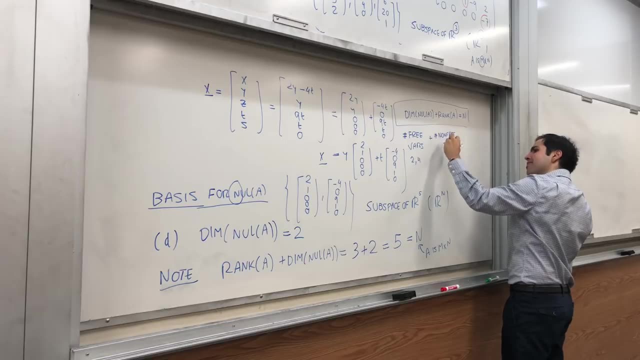 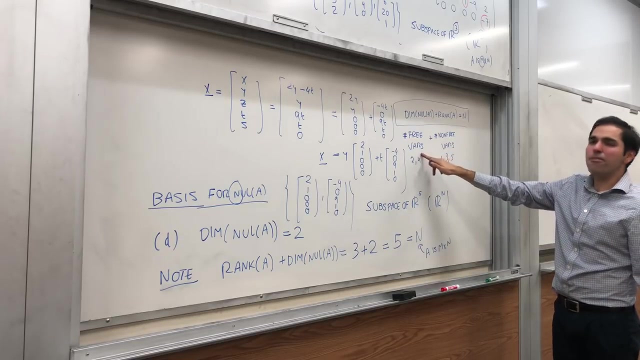 You know. so here were- it was, like you know, columns two and four, plus number of non-free variables, which were columns one, three and five. Well, if you add the number of free variables and the number of non-free variables, 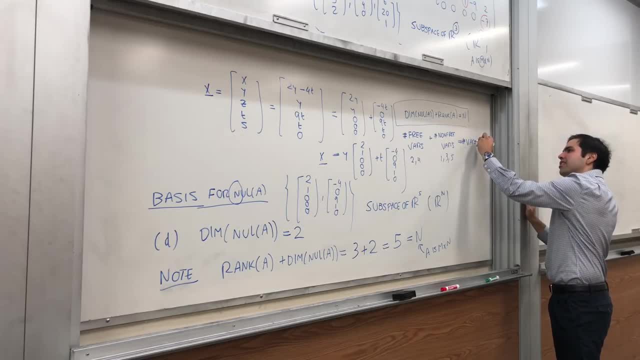 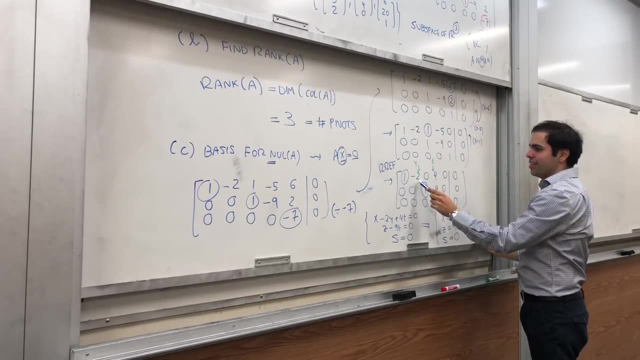 you get the total number of variables, which here is five. So in fact, you see, if you add, you know. so add all the columns together. so the free variables were in columns two and four, the non-free ones are in one, three and five. 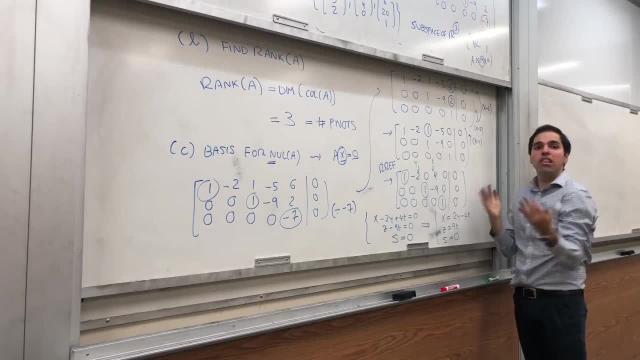 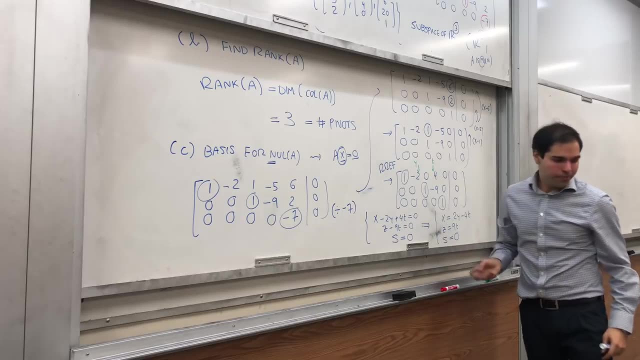 Well, the total number you'll see now is just the total number of columns. That's why we do n, We don't do m, because that's the number of rows. Okay, that's all I wanted to talk about here, okay. 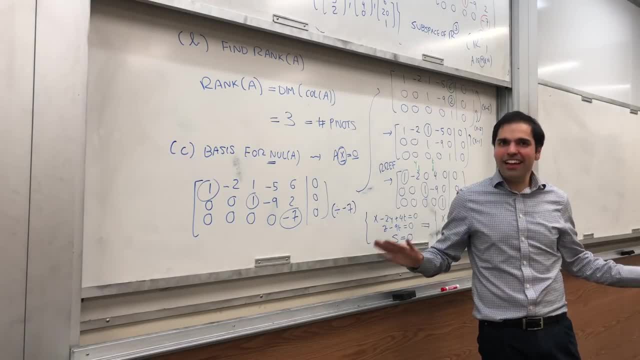 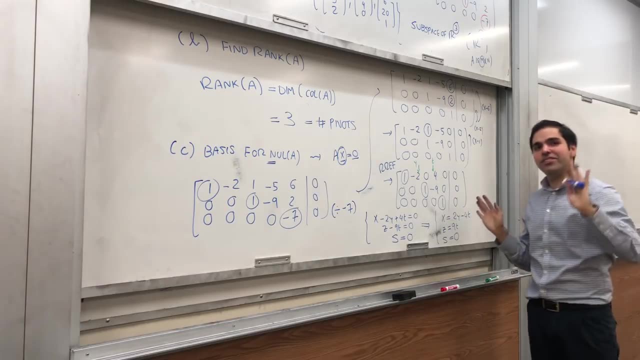 So if you're taking my class, at least Math 3A at Irvine, this is, you know, the stuff we care about. Just in case you're taking more than that, just the row space. let me talk a little bit. 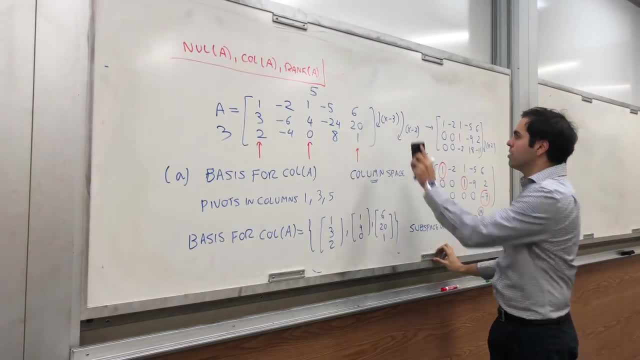 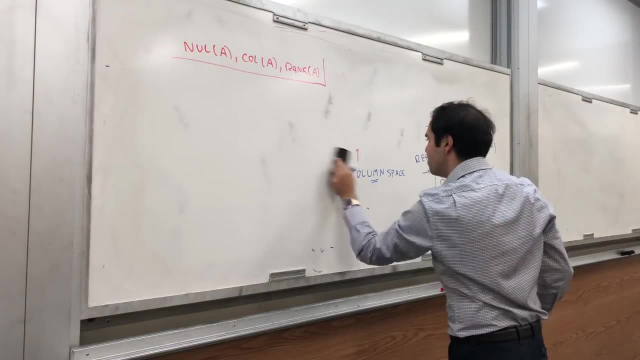 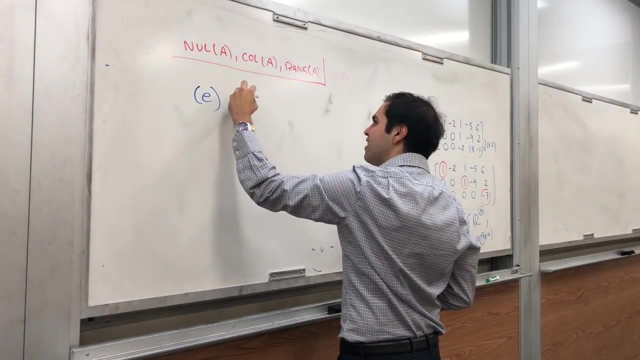 about the row space. So again, let's take this matrix and find a basis for the row space of A. It turns out it's even easier- So I think it was number E or something- Find a basis for row of A. 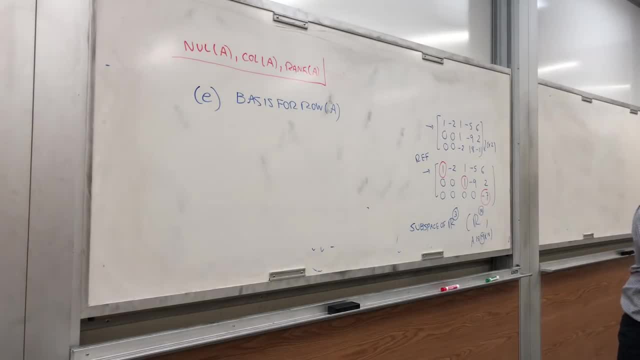 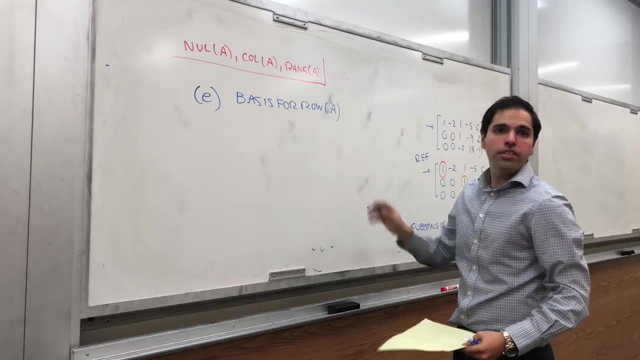 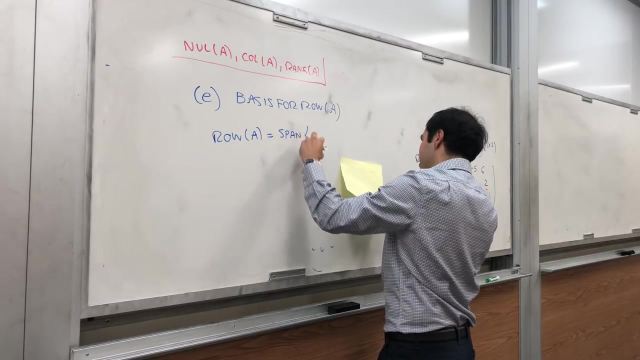 Now, fortunately I raised this matrix. but what the row space is is simply: you take all the rows as vectors and you take the space and the span of it. So here row of A would be the span of three minus. sorry, wrong matrix, sorry. 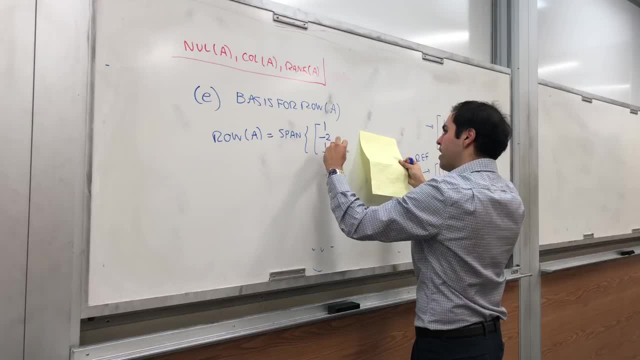 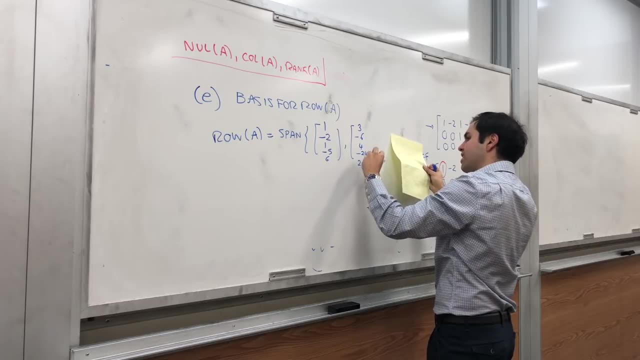 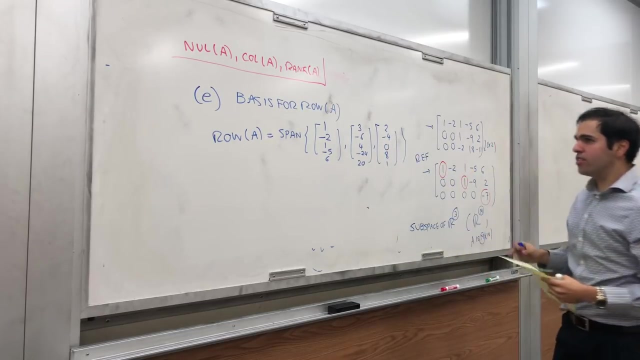 one minus two, one minus five, six and three minus six, four minus 24,, 20, and two minus four zero eight one. That's a row space, and it turns out. the nice thing about the row space is: 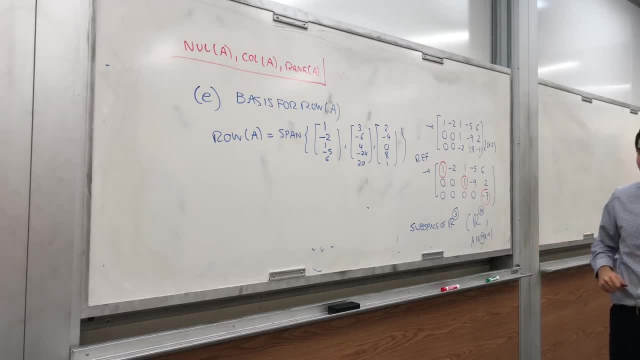 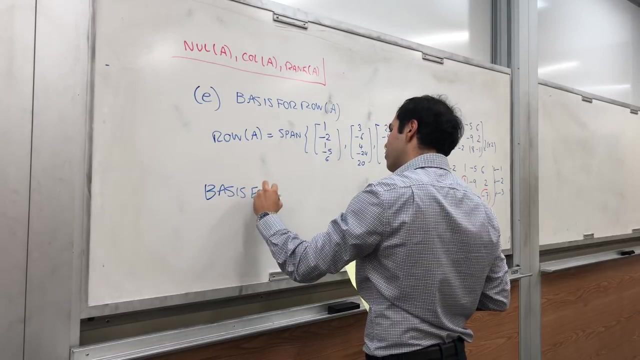 in order to find your basis, you don't need to go back to the original matrix. Just see in which rows the pivots are. Well, the pivots are in rows one, two and three. So indeed, a basis for the row space of A. 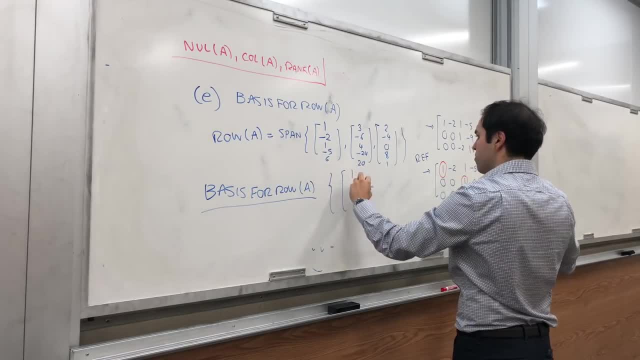 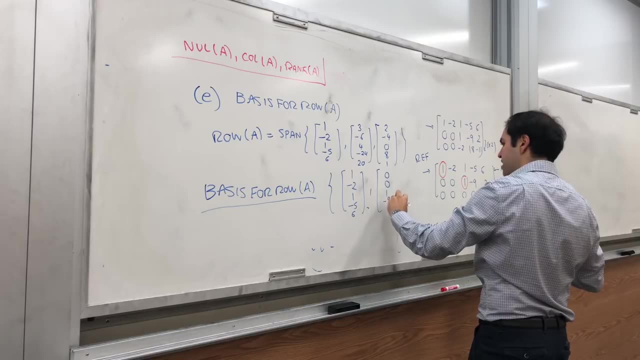 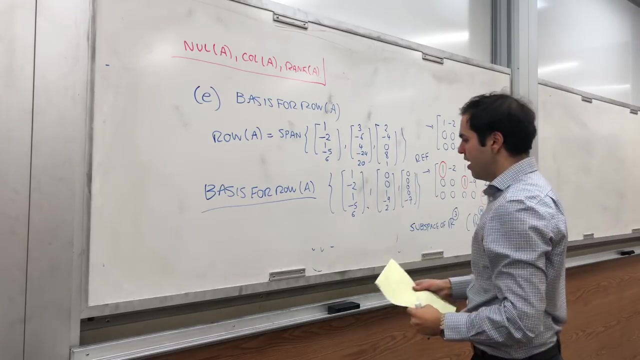 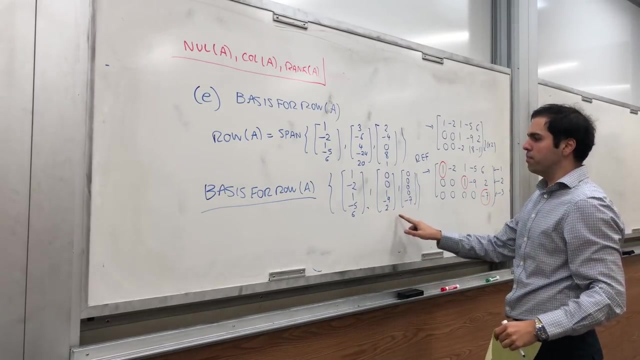 are simply your new vectors. So one minus two, one minus five, six zero zero, one minus nine, two and zero, zero, zero, zero minus seven. And here notice the row space. In this case it's a subspace. 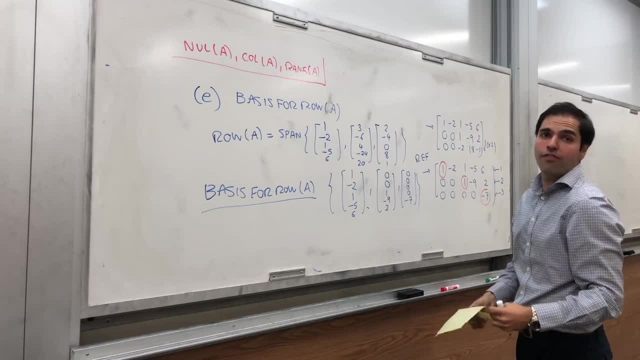 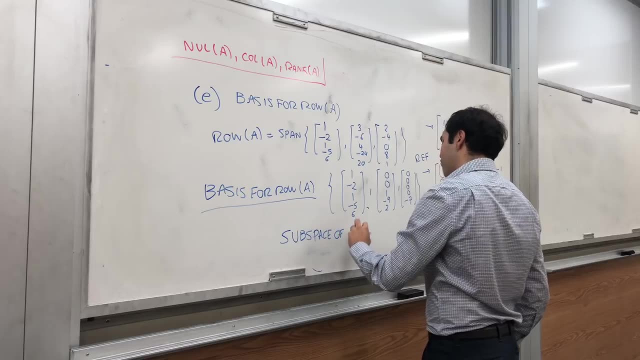 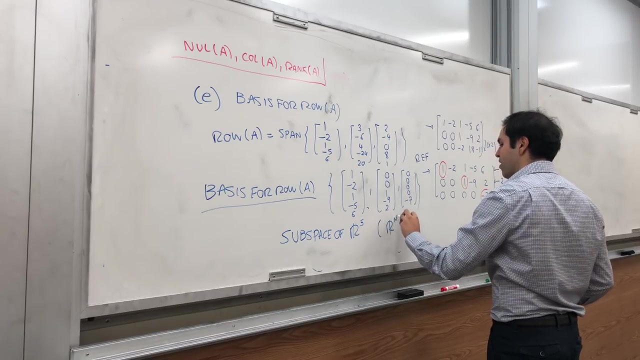 you know, like each component has, each vector has five components, so it's a subspace of, you know, R five here, which in this case it's N. So in general it's a subspace of R M. 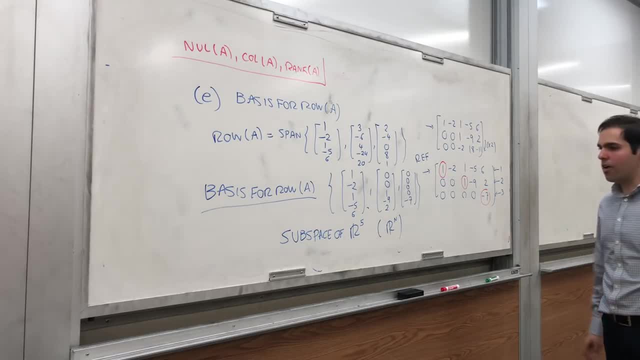 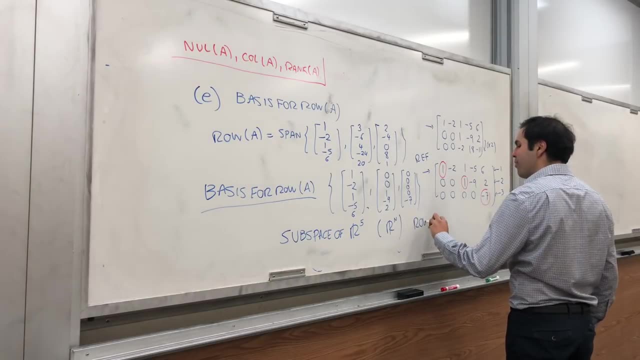 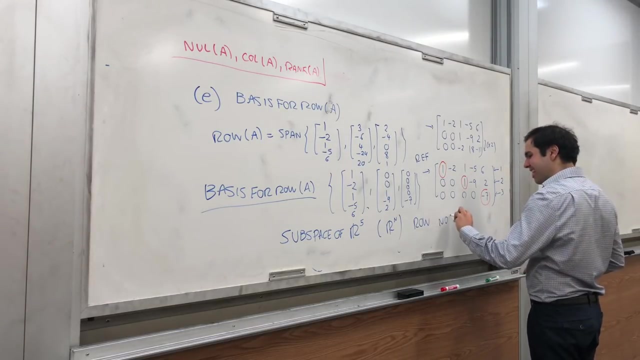 Okay, Where it's careful. the column space was a subspace of R M and I don't know how to remember that. but one thing is: maybe row row sounds like rows, like nose. That's why it's a subspace of R N. 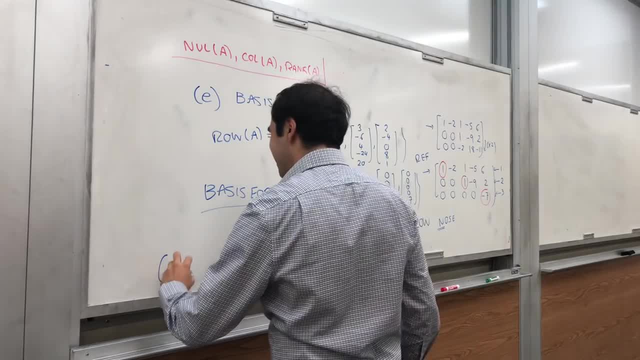 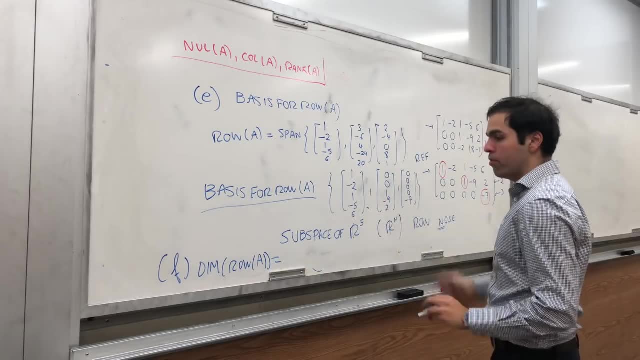 I don't know. Okay, Lastly, just then, what is the dimension of row of A? Well, the nice thing is, we found the number. you know, we found a basis. just count the number in the basis, which is three. 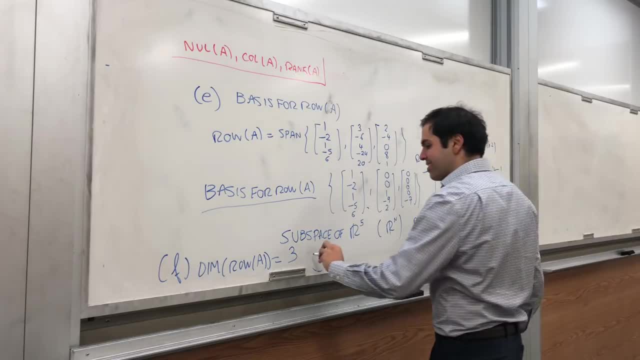 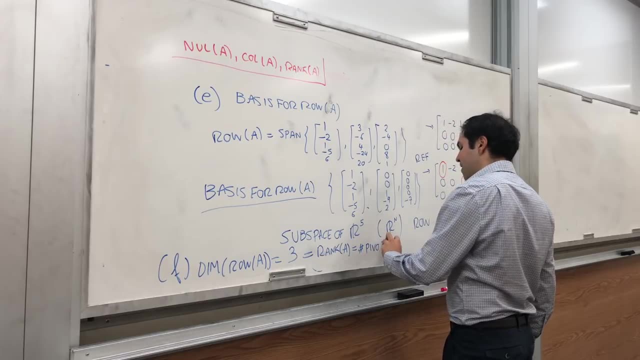 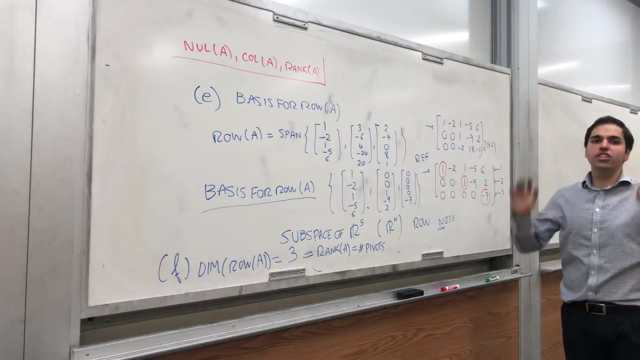 and it turns out, incidentally, that's the same as the rank of A, because that's just the same as the number of pivots. So, even though the row space and the column space are two different things, the dimensions are the same. 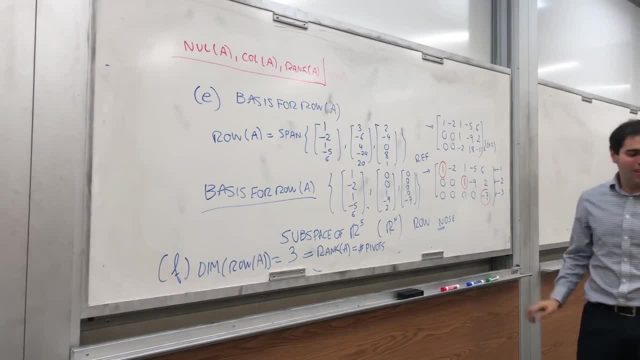 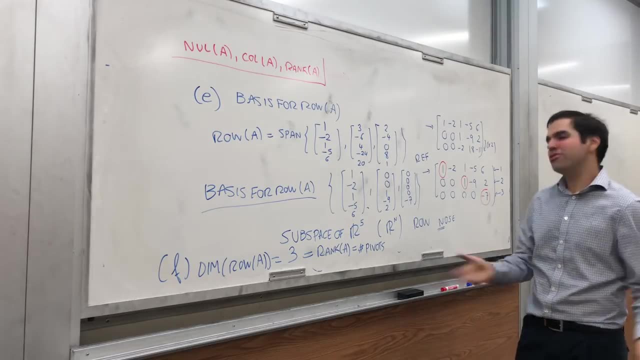 which is a bit surprising, but I think it's pretty cool. And also, why don't you have to go back to your original matrix? Because row operations are nice. with rows, They preserve span and linear independence, So it gives us an easier basis. 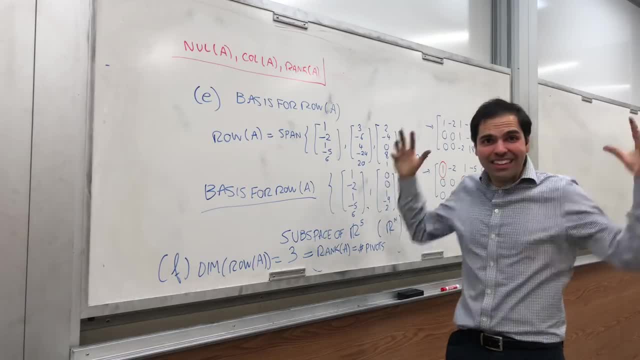 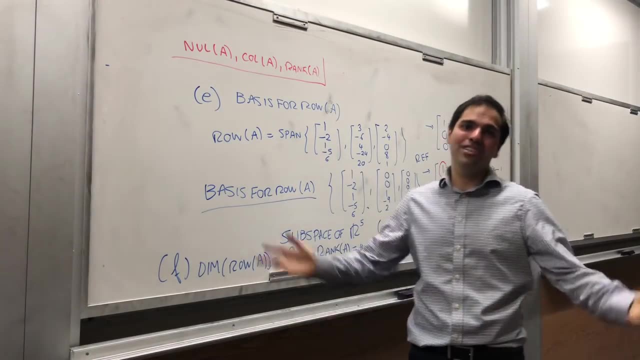 if you like, All right. So I hope you like this linear algebra craziness Extravaganza. If you want to see more math, please click like and make sure to subscribe to my channel. And yeah, I think it's time to go.